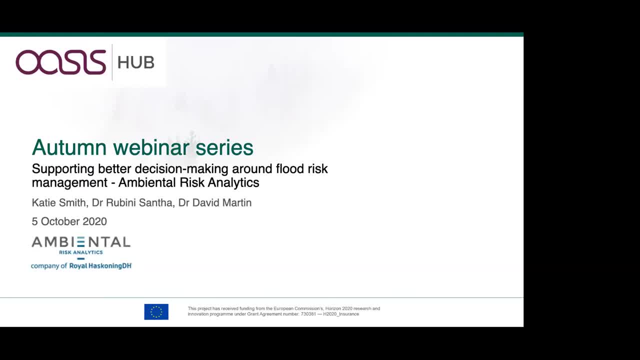 bit about some of the challenges that you need to address. You can see the details of our other flood webinars that are coming up and the one you might have missed. I'll post the link in the chat box shortly, but today we're going to present a really exciting set of digital services provided. 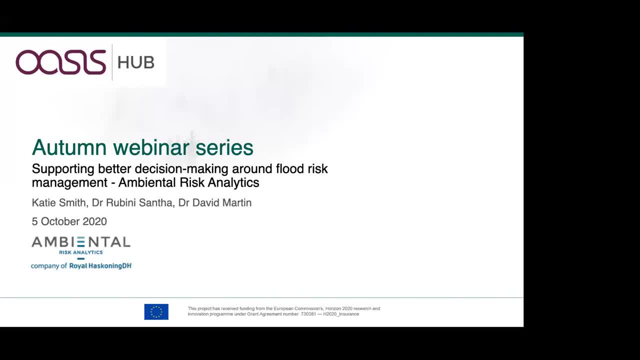 by flood, specialist Ambiental Risk, which can support you in addressing global flooding challenges and flood risk. We're about to see presentations of three separate services, the first from Katie Smith, who's a technical manager at Ambiental and a senior member of the flood modelling team. 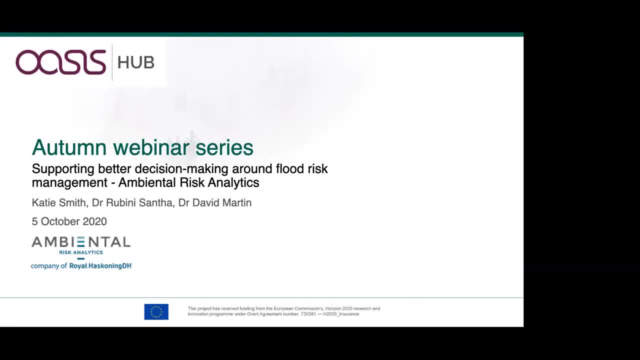 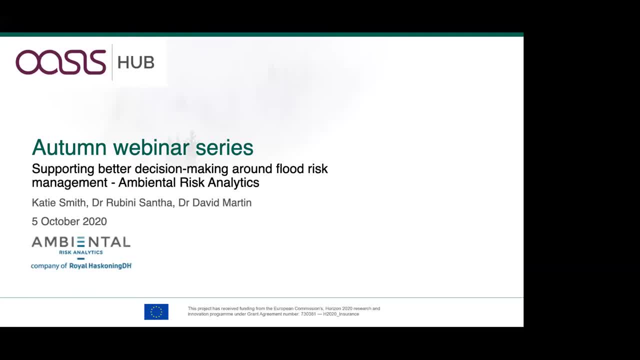 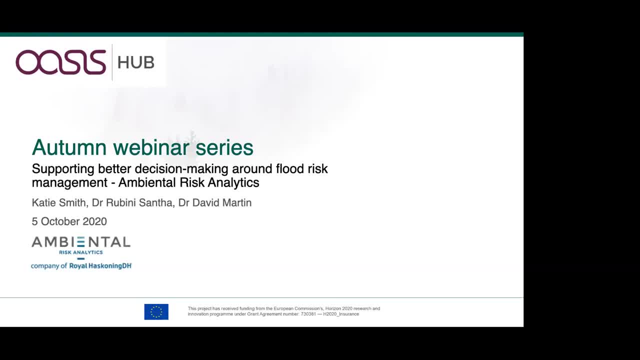 which is a predictive flood model that considers nine possible climate change scenarios between 2020 and 2080, and this is aiming to help insurers and reinsurers, utility companies, local authorities, infrastructure managers, commercial developers and others understand and plan for long-term flood risk. 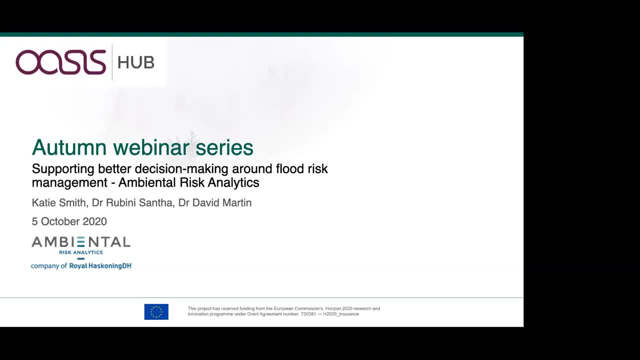 and others understand and plan for long-term flood risk. Our last speaker will be Dr Rubini Santha, who's a lead catastrophe modeller, flood cap model developer and an expert of lidar remote sensing for hazard mapping applications. They're going. 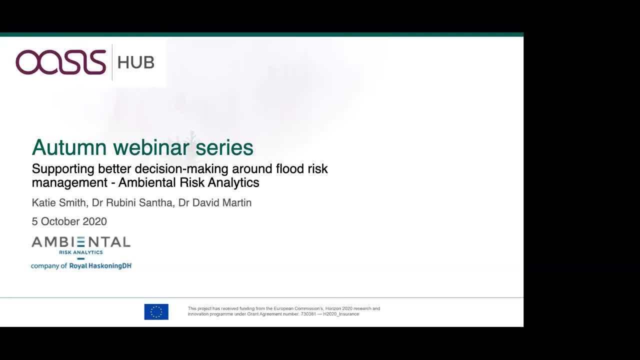 to present FloodCat, which are models which use historic river rain and tide gauge data to simulate potential future flooding disasters. I'm going to take questions after the three presentations have been made, but please feel free to post them in the Q&A or chat boxes as we go. 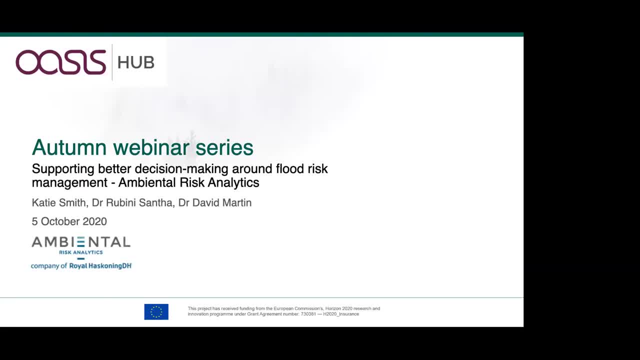 along Before we hear from the speakers. I'm going to hand over to Rob Carling from Ambiental Risk, who's going to give you a quick introduction to the company. As Will said, I'm going to hand over to Katie Smith in a few minutes, just on the European. 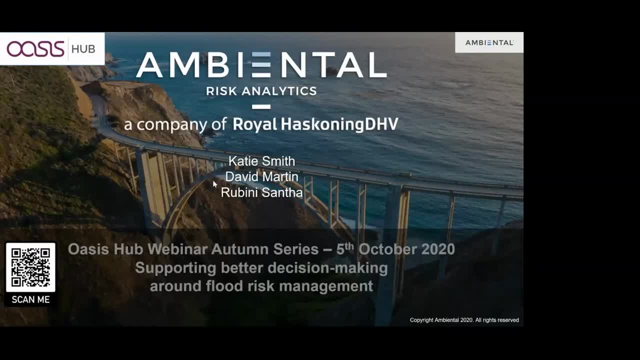 data, then David, then Rubini, Just really a little bit about Ambiental as well. There is a scan me code, you'll see, and also we're offering an exclusive offer of a consultancy sort of review as well. So that would be at the end of the presentation and, as we all said, 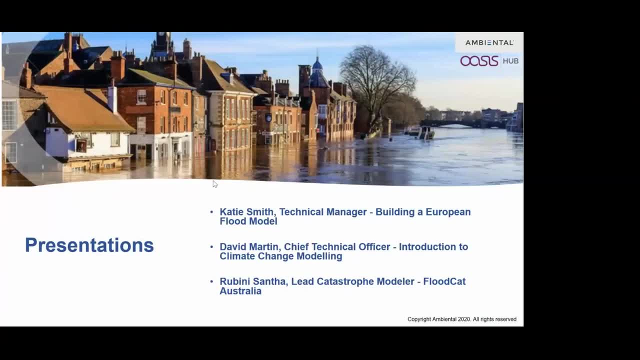 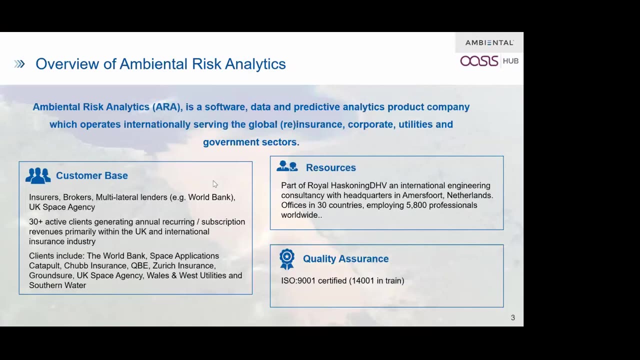 we'll take questions at the end. Just a really little bit as Will introduced. these are the three speakers- I hope you can see the screen there: Katie Smith and David. then Rubini. Really just a little bit about Ambiental. We're dating back to 2001, 2002.. We're specialists in 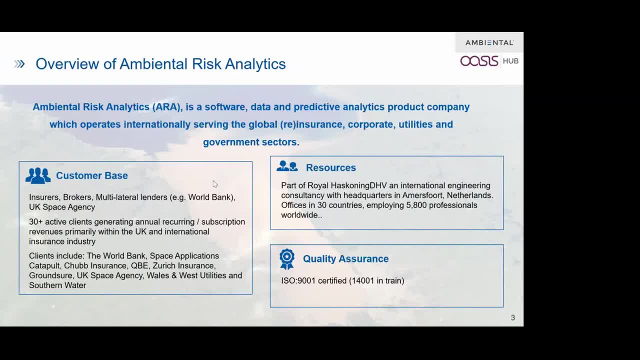 flood, particularly in the insurance and financial sector, with the UK, European and globally. We have national scale sort of flood models and some of our clients include the World Bank, the Space Application Agency, the Chubb Insurance, QBE, Zurich and many, many more. 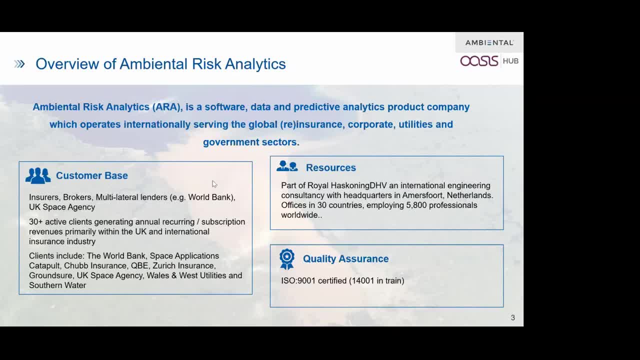 We were recently taken over- well, probably 14 months or so ago now- by Roar Haskell, a global consultancy, Dutch consultancy. over 6,500 colleagues across the globe, in over 30 countries. We're quality assured as well, so everything we do is quality assured and sort. 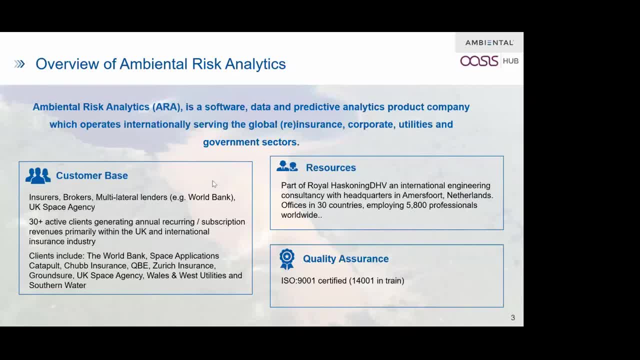 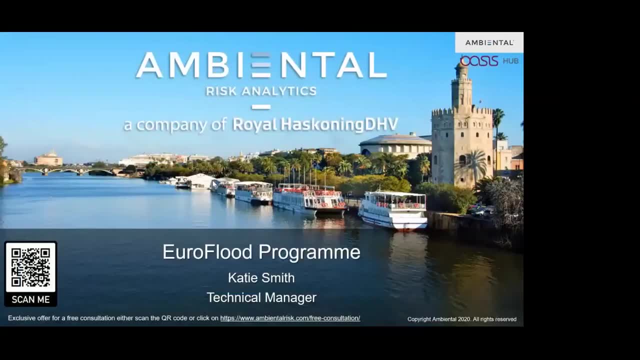 of tested. So, with more to do, I'll just hand you over to Katie to start with, and I'll be back at the end to sort of go through a sort of wrap-up as well. Thank you, Over to you, Katie. 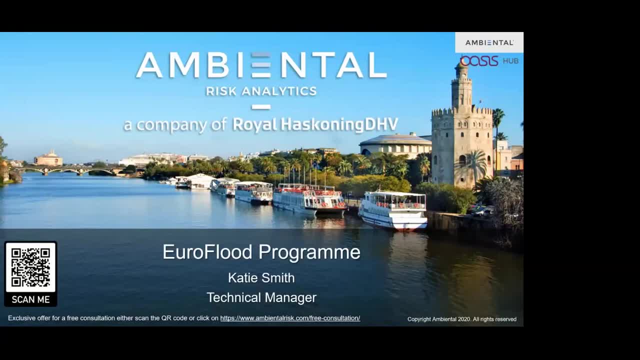 Thank you very much, Rob. Yes, so, as in introduced by both William and Rob, my name is Katie Smith and I'm a technical manager at Ambiental, having worked for the company for about five years now. But yeah, so today I'm. 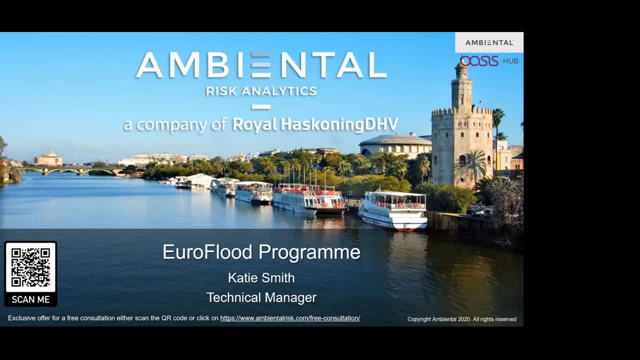 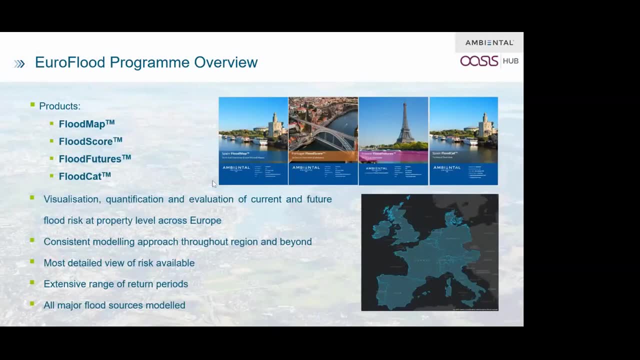 going to talk to you about our Euroflood programme. So, Rob, if you could go onto the first slide please. Perfect. So our Euroflood programme comprises the development of a new suite of flood risk products, including Floodmap, Floodscore, Floodfutures and Floodcat. 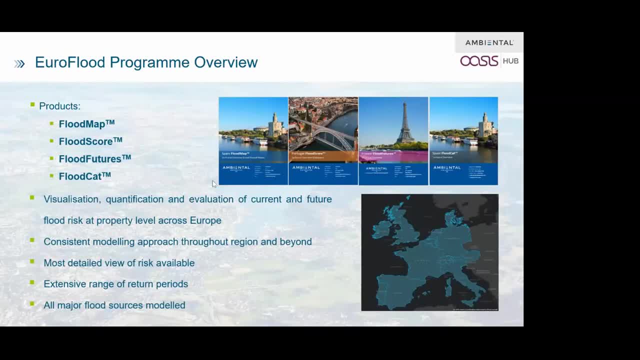 Which we are currently rolling out in countries across Europe. We have applied the same modelling techniques as those employed for our existing flood risk solutions in other territories throughout the world, thereby creating a globally consistent view of flood risk. Together, these products allow customers such as insurers, utility companies, 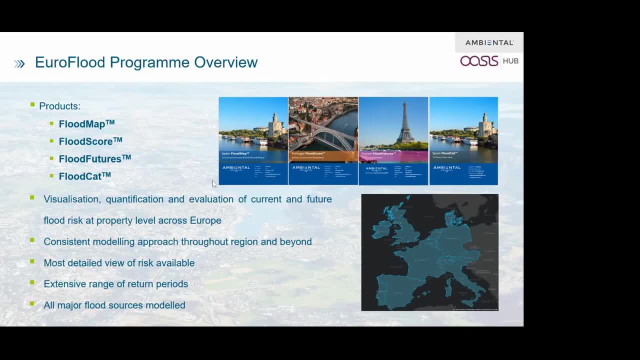 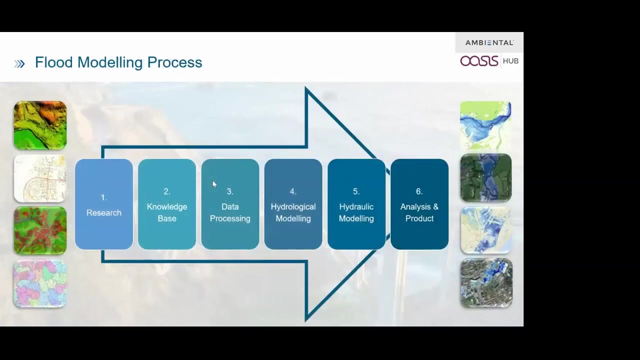 local authorities and risk managers to understand and assess the current and future flood risk to their assets or exposures. Today I'm going to focus on our Euroflood Floodmap and Floodscore product, with my colleagues presenting to you Floodfutures and Floodcat. So could we move onto the next slide, please, Rob, Thank you. So firstly, I wanted to 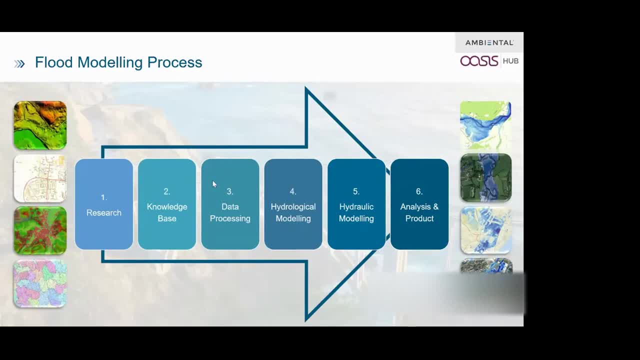 provide an overview of how we approach flood modelling at Ambiental. So whenever we initiate a project in a new territory, we follow this process, which starts with a research phase and ends with a final flood hazard mapping product. One of the first steps is to go. 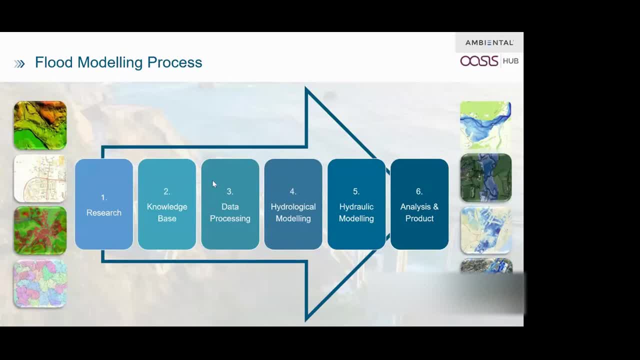 and conduct extensive research to gain an understanding of exactly what data and information is already available and how we might develop a flood model in this territory. We obtain this information from a range of sources, including government agencies, data suppliers, academic literature, media reports and so on. Once this phase is complete, 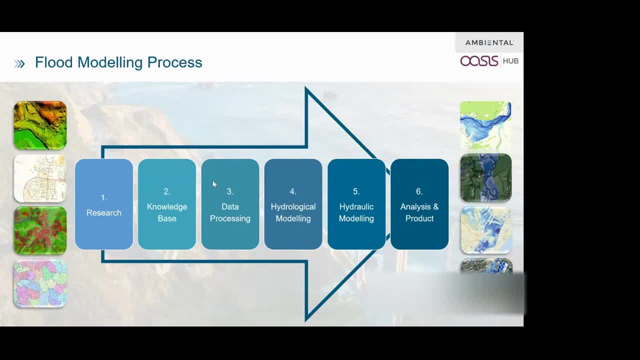 we then start to build our knowledge base of the various input data sets required to support the hydraulic modelling. These data sets include geospatial layers such as topography data, for example, digital terrain models or DTMs, gauge data, land cover data and also information about flood defences. 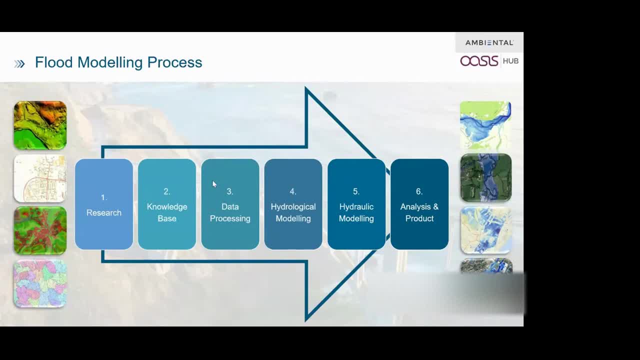 The next stage involves the analysis and pre-processing of the numerous input data sets using GIS, to enable that everything is in a correct and compatible format. So this process includes treating the data to remove artefacts that could potentially unrealistically impact the results of our hydraulic modelling, for example. 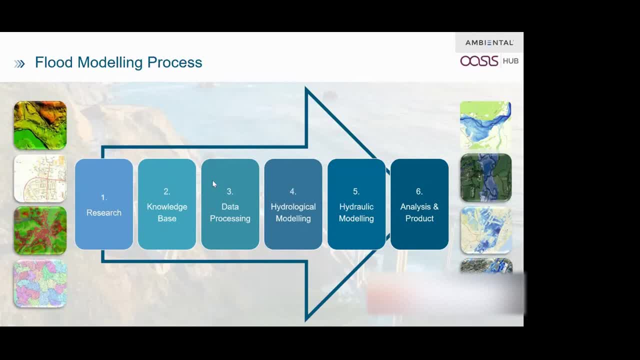 and it can also include aligning the format and resolution of data sets from a range of different sources. Hydrological modelling is then performed to calculate the flood model input, river flows, rainfall intensity and tidal levels. In the case of our Euroflood product, we have used local 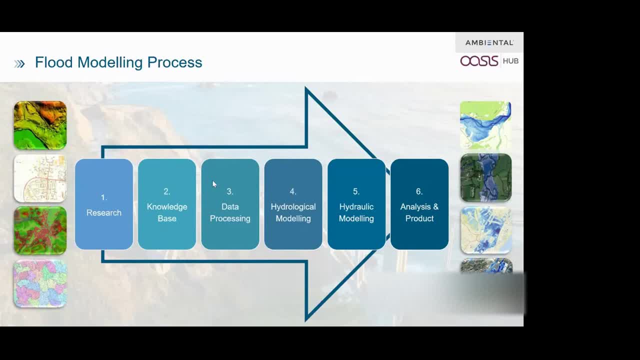 hydrological methodologies and parameters within each country that we've modelled. So then, moving on to the hydraulic modelling, So everything that has been processed and obtained up to this point is then used as inputs to the hydraulic modelling, which involves running hundreds of thousands of overlapping flood simulations, the outputs of which 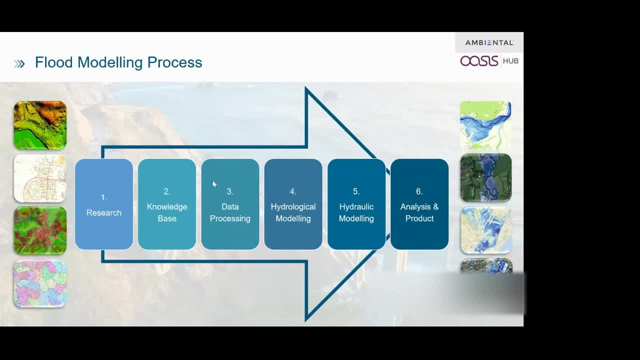 are combined to form our flood hazard maps. For Euroflood, we used our own proprietary 2D flood modelling software to do this, FlowRoute Eye. So then, finally, once the flood hazard maps have been built, they are subject to rigorous quality assurance inspections, both automated and manual, in order to validate the modelled outputs. 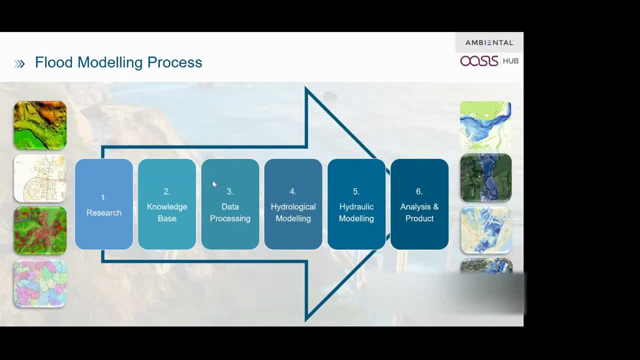 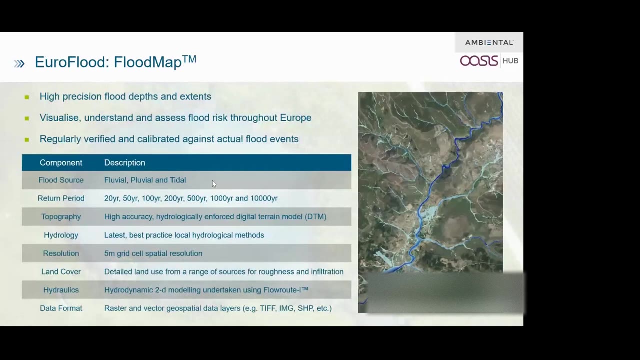 The flood maps are also regularly verified against real flood events, events which are identified as part of the research phase. So if we could move on to the next slide, please, Rob. Thank you. So now I'd like to explain our Euroflood flood map products. 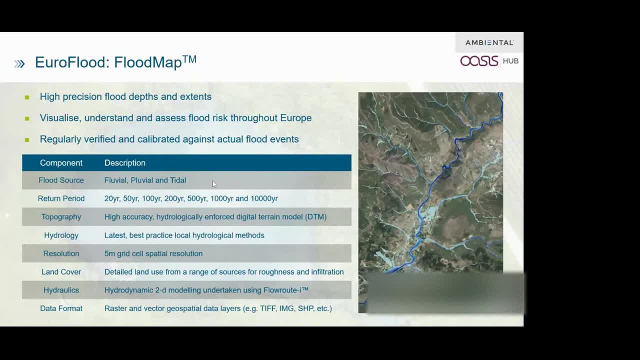 in a bit more detail. So these products provide high precision flooding depths and extents at five metre resolution for a range of return periods from the 20 year up to the 10,000 year for multiple flood sources, including fluvial or river. 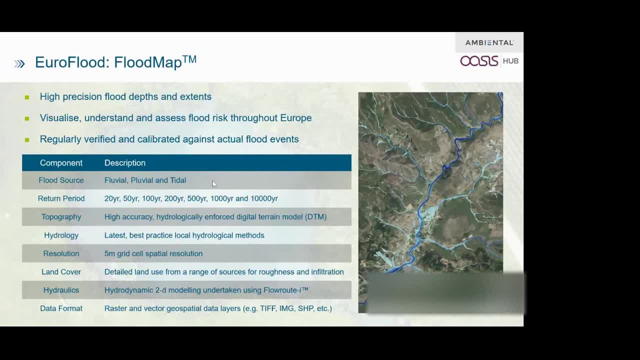 pluvial or surface water and tidal or coastal storm surge flooding Flood map is available at a national scale for countries in Europe, having been developed using a high resolution pan-European VTM and our globally consistent modelling techniques, with the increased accuracy benefits of incorporating local sub-country. 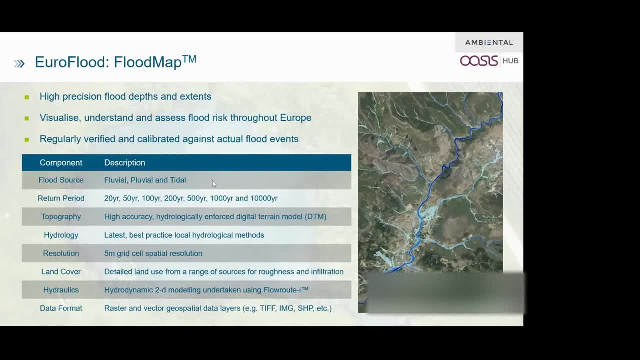 or hydrological parameters and methodologies. Ultimately, our flood map products provide customers with the ability to visualise, assess and understand flood hazard where it matters to them. And the image on the right hand side there is just an extract of our Spain pluvial, so our Spain surface water flood. 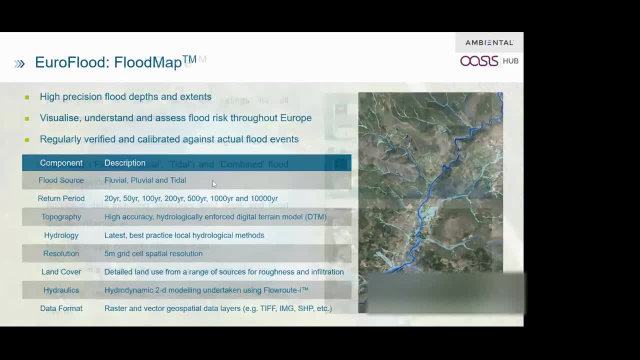 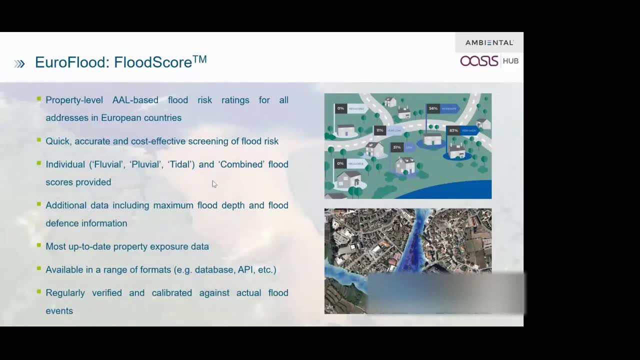 map So we can move on to the next slide. please, Rob, Thank you. So now I wanted to talk a little bit about our Euroflood flood score products. So these products provide flood risk ratings for all properties in European countries, covering 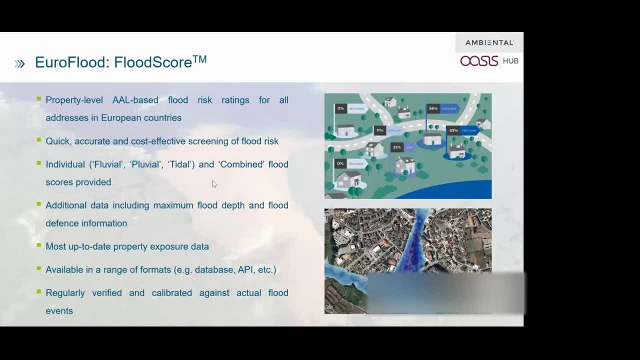 both residential and commercial premises. Flood hazard depths are extracted from our flood map data to each individual address and combined with unique damage values to produce average annual losses, which are then scaled into flood scores of zero up to 100.. These risk ratings are also classified into bands from negligible up to 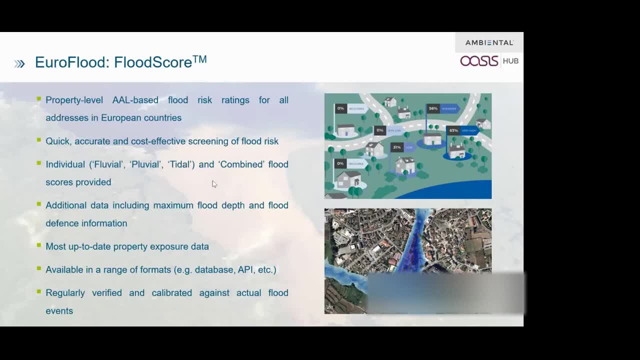 very high and are consistent both within and between countries in Europe and beyond. For each individual property, a combined risk rating is provided in addition to individual scores for each flood source. So essentially, flood score gives a measure of the likelihood and severity of flood risk at the property management level. The flood 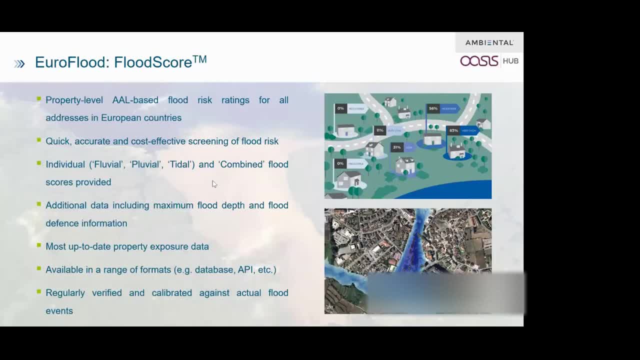 level, and it also includes supplementary information, such as the maximum flood depths for all modelled flood sources and return periods, And also other metrics are available, such as annual damage ratios, which are relevant to the insurance sector. And finally, the last thing I was going to say about flood score here was that 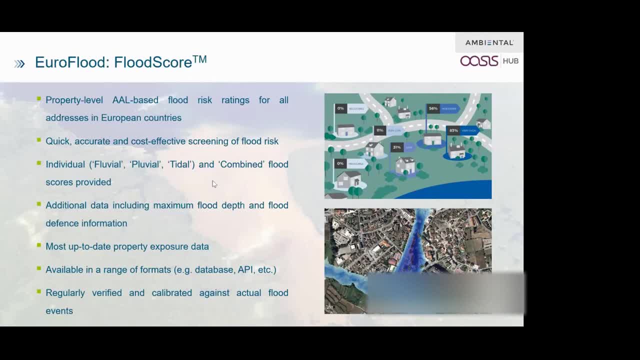 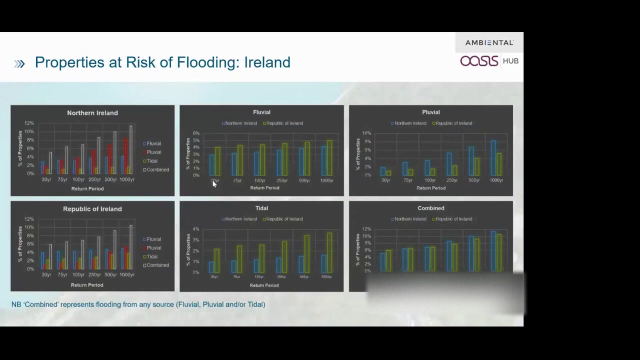 it facilitates the screening of exposure portfolios and supports decision making by enabling risk thresholds to be established, For example by deciding to only ensure properties with a flood score up to 50. That's how a lot of companies use our flood score datasets. Thank you, Rob, And so yes, now moving on to the next slide. I just 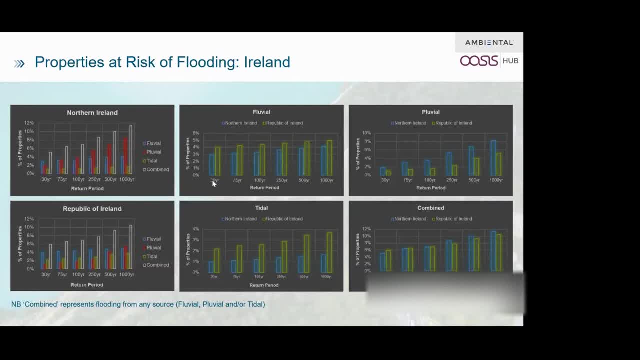 wanted to show you examples. We've got some examples of some insights and comparisons that can be derived from our Euroflood flood score databases, The first of which shows breakdowns of the percentage of properties at risk of any depth of flooding in Northern Ireland and the Republic of Ireland. firstly, by 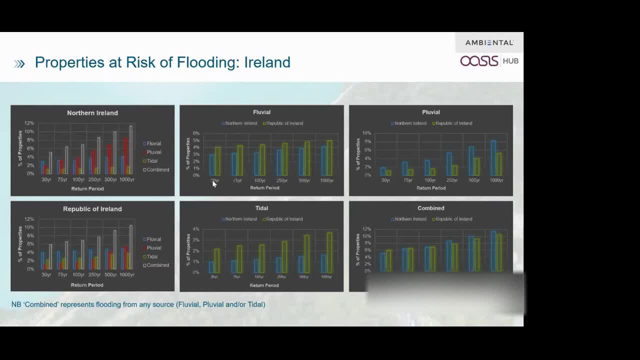 region and then by flood source. So, in terms of the proportion of total properties affected, the combined chart, which you can see on the side, shows us that both Northern Ireland and Republic of Ireland experience similar levels of risk. However, by looking at the other graphs, the data shows us that this risk is driven by: 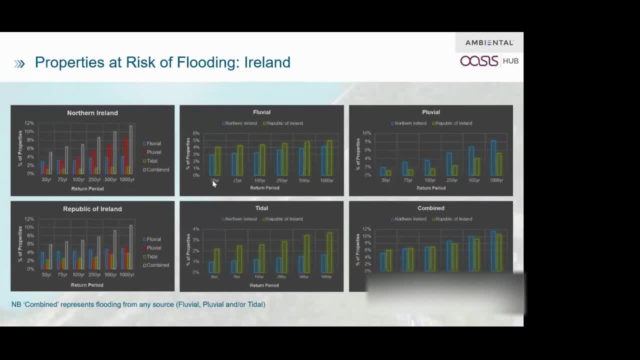 different flood sources. In the Republic of Ireland, fluvial and tidal flooding affect the greatest number of properties, whereas in Northern Ireland, pluvial is the dominant source of flooding. In fact, according to the Department of Infrastructure's Flood Risk Assessment, 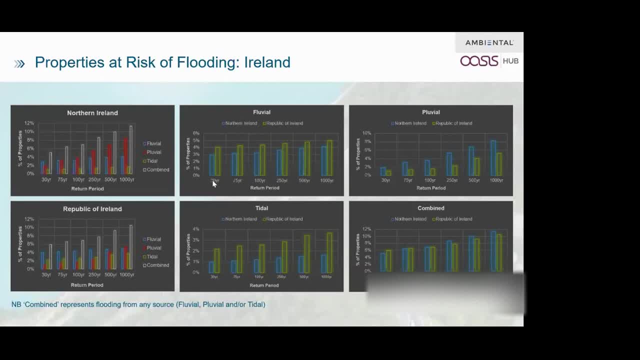 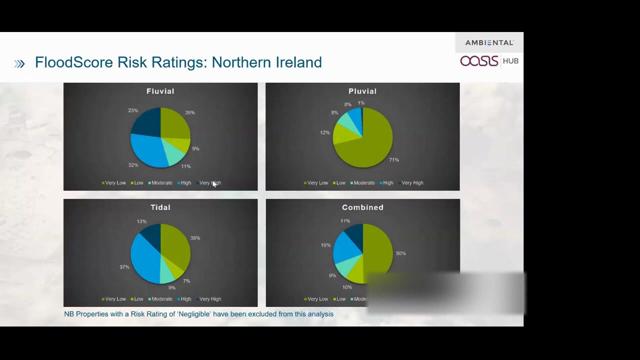 Northern Ireland is actually estimated to have aggregated annual average damages of £56 million, 74% of this actually being attributed to pluvial flooding. Next slide, please, Rob. Thank you. So, in contrast to the previous slide, which looked only at the 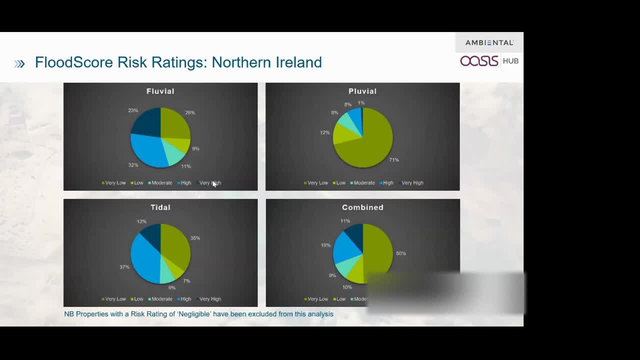 amount of properties affected by any level of flooding. these charts represent the distribution of flood risk. So, in contrast to the previous slide which looked only at the distribution of flood score, risk ratings between very low and very high and therefore include estimations of likely damage. So, overall, half the properties within these risk bands in Northern 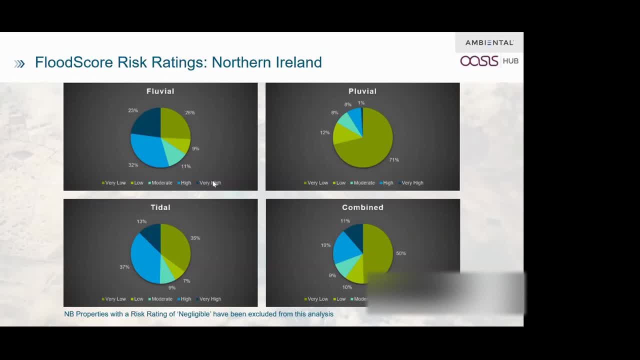 Ireland are classified as having very low flood risk, And although we can see that the majority of properties affected specifically by pluvial flooding are calculated as having very low risk, there are many more properties affected in absolute terms, which is why it is the most. 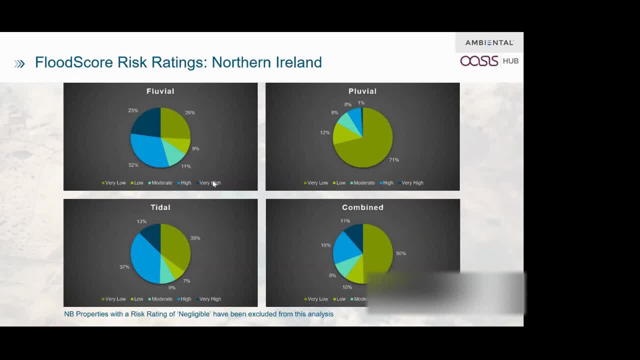 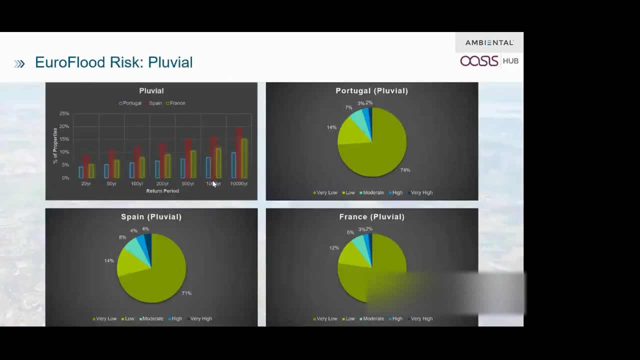 dominant flood risk in this region. And on to the next slide, please Rob. Yes, so this is just a final example, but this time focusing specifically on pluvial flooding across Spain, Portugal and France. So, in terms of the proportion of total properties affected by, pluvial flooding, there are many more properties affected in absolute terms, which is why it is the most dominant flood risk in this region. And on to the next slide, please Rob. Yes, so this is just a final example, but this time focusing specifically on pluvial flooding across Spain, Portugal and France. So 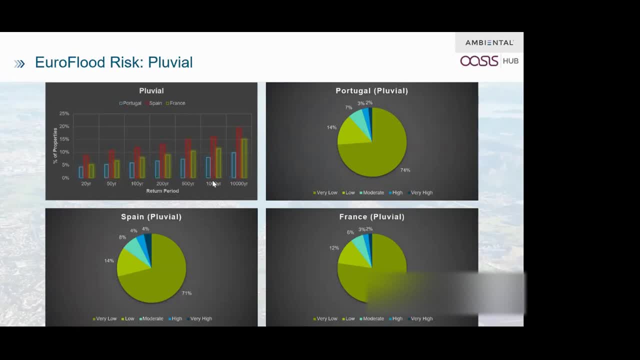 in terms of the proportion of total properties affected by pluvial flooding in each country, Spain is shown to experience the highest, while Portugal experiences the lowest. These graphs also show us the distribution of risk within our flood score risk rating categories, And it shows us that it's. 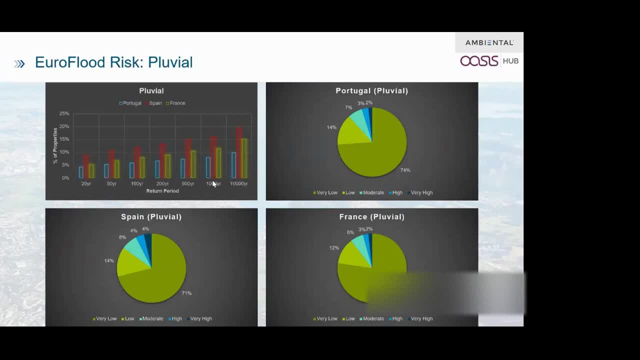 very similar actually for each country, And the reason I wanted to show this is that our flood score databases- from you know, different countries can be compared to each other, And so we've used the same modeling and approaches, And also our risk ratings are truly linear, And so 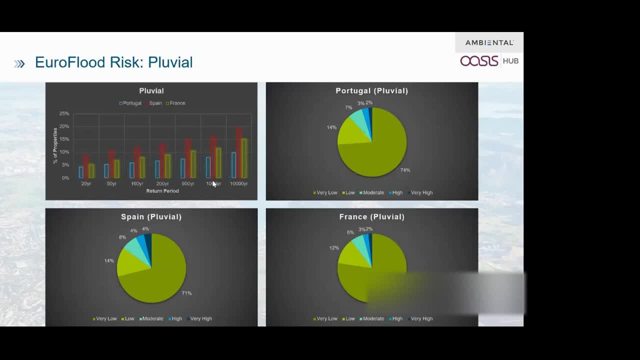 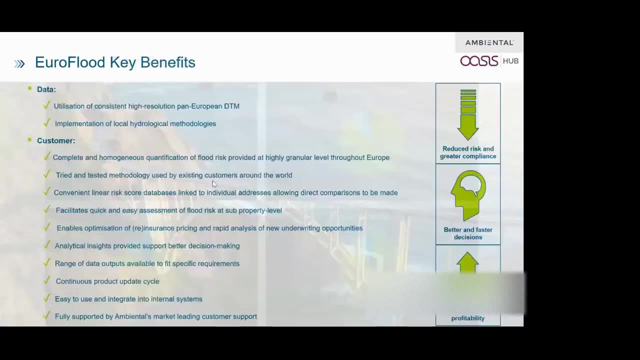 therefore, a score of 50 is exactly half the risk of a score of 100.. On to the next slide, please, Rob. Thank you And yes. so finally, I just wanted to discuss and kind of recap on some of the key. 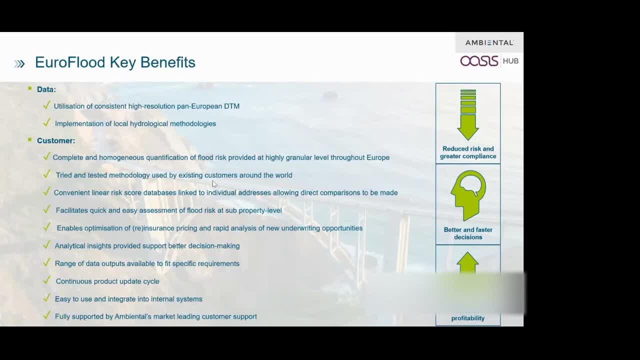 benefits of using our Euroflood flood map. Yes, so finally, I just wanted to discuss and kind of recap on some of the key benefits of using our Euroflood flood map and flood score products. So our Euroflood products include multiple flood sources and return. 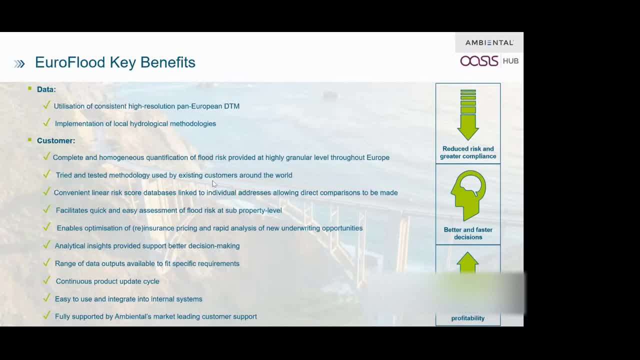 periods which provide a comprehensive and complete view of all major types of flooding for countries across Europe. The analytical insights we provide support better decision making around flood risk management by predicting the location and severity of flooding, preventing damage and protecting people, property and assets. 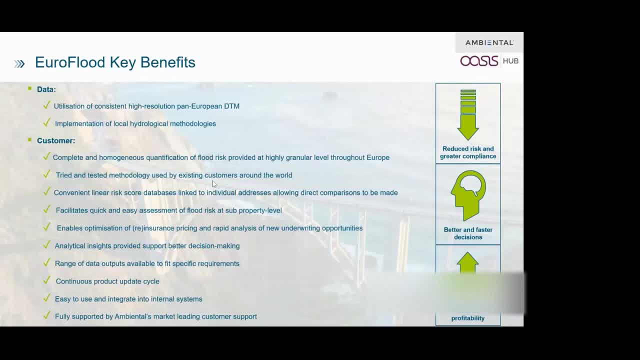 We have incorporated the most accurate European wide, high resolution DTM, the benefits of which include uniformity in the specifications and characteristics between countries. And although local models certainly have value, they often adopt different approaches and cover small areas and are therefore insufficient for fully understanding hazards and underwriting flood risk across entire countries. And so we've incorporated 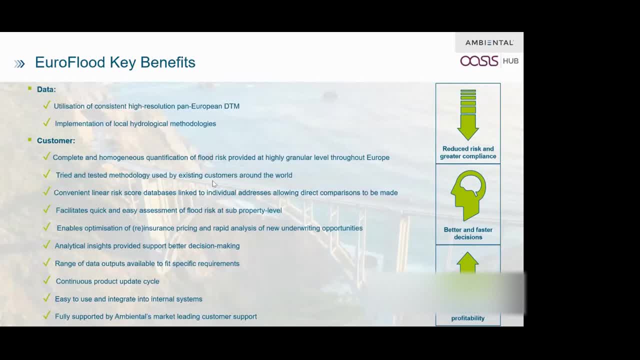 more ratios to help change flood risks depending upon the local and national pattern. But our Euroflood products, however, are created using consistent modeling frameworks but with localized hydrological methods and parameters which allow Austral stomach also arguments. let us see how water seventy thousand different. 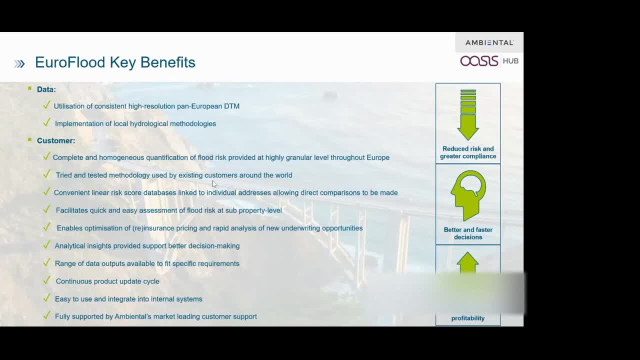 zin fib Bravo located in Ziel ashamedro AB Pr. Vacavius, which allows us to ensure the highest possible accuracy and precision at very large scales. Destination لاüman MPH. This allows end users to compare the risk both within and between different countries and throughout the 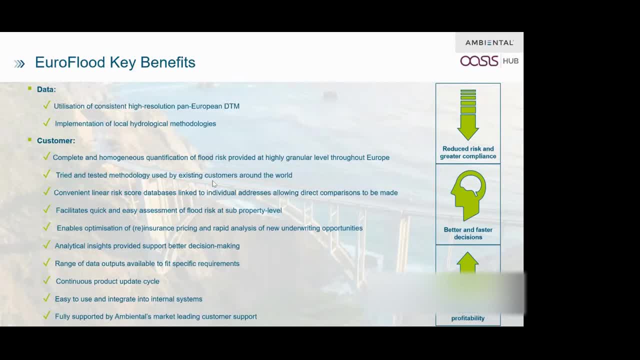 world. as the Final, Finally, I have a flood. products are available in many specific countries across Europe and colas�� āh. We have a range of formats to align with specific end user requirements and are also supported by detailed technical documentation, so customers are confident in their understanding of the data. 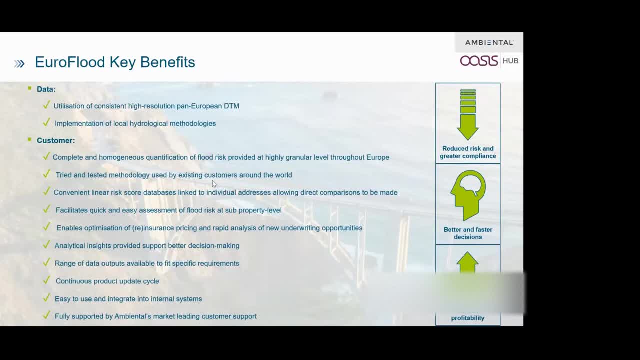 We also have continuous product update cycles for future enhancements, including the integration of high precision LiDAR, And change reports are also supplied with each of these updates, which clearly explain any alterations that occur to the hazard and or exposure. Thank you very much for listening. 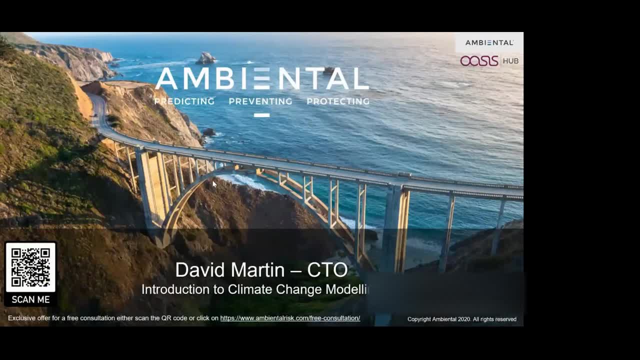 Thank you very much, Katie. That's a really great presentation and good overview of our flood school. As Will mentioned, there's an opportunity for questions at the end of that. Next I'm going to pass over to my colleague, Dave Martin. 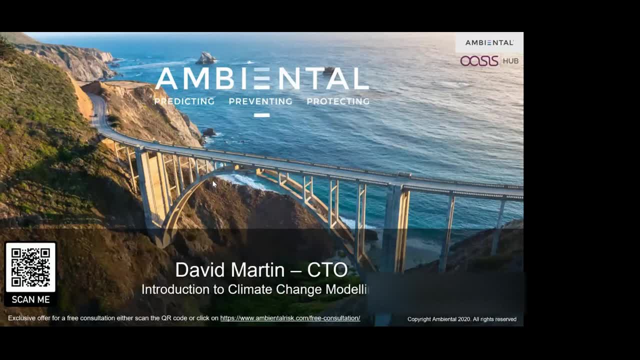 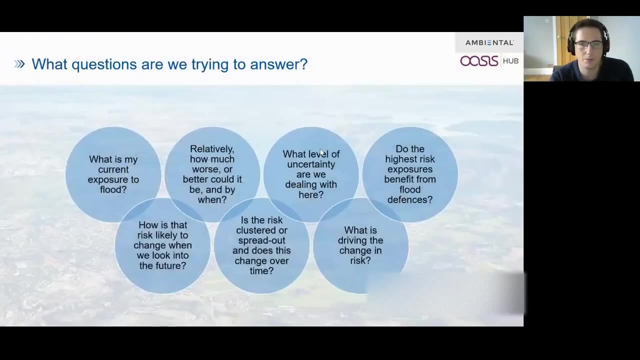 He's going to look at the introduction to climate change modeling Over to you, Dave. Thanks, Rob, Can you hear me? OK, Yes, we can. Yeah, Excellent, Brilliant, OK, cool, Yeah, Do you want to just pop on to the next slide? Wonderful. 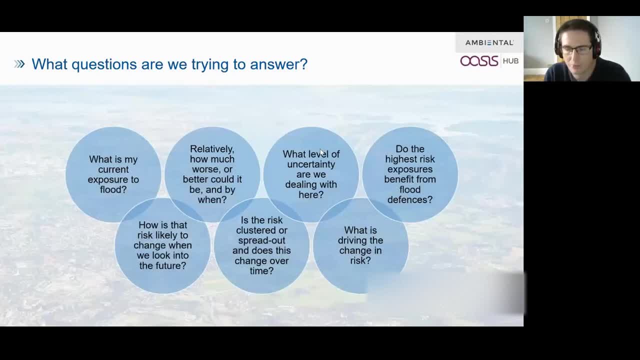 So I'll spare the introductions because I've got quite a few to get through, But OK, so I'm going to talk about climate change, modeling and flood for a bit, And it's tricky. When we talk about climate change, it's probably a good idea to first think about why. 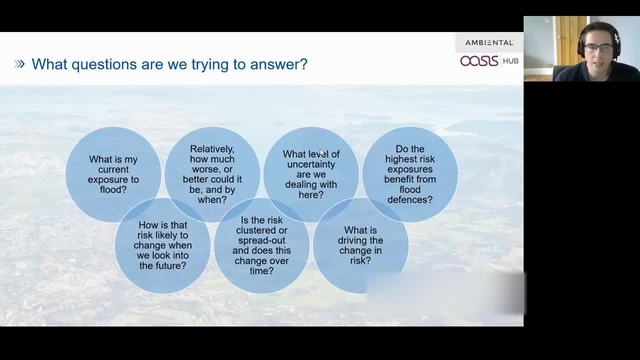 What are some of the questions that we're looking to answer Now? climate change, for me at least, is a question of sensitivity. It's a question of trying to understand the uncertainty over the future and perhaps narrow down what the parameters are relevant to, whatever it is. 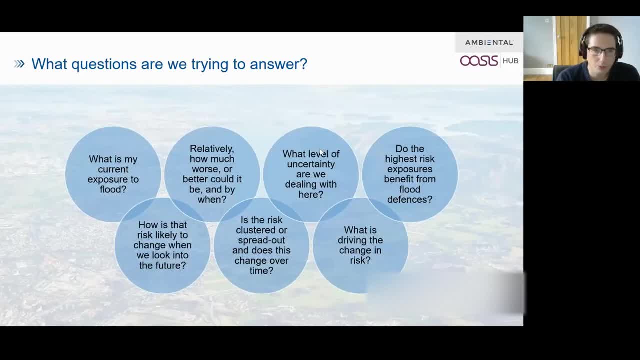 we're concerned with whether that's an insurance portfolio or pipelines to manage properties, to plan Ultimately. we're trying to answer the question: do I or should I consider changing my strategy to flood risk now because of what might happen in the future? 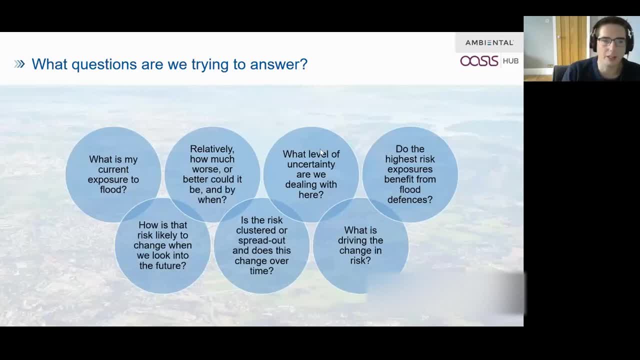 So the thing with flood is it's inherently a very granular problem. The risk to your neighbor's house Can be completely different to the risk to yours. It's probably not, but it can be. So climate changes and the impact of that, how climate change can change the frequency of these sort of things, can have impacts on a very fine scale. 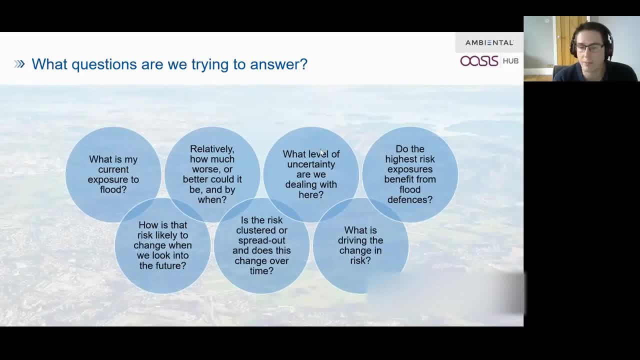 So we think it's beneficial to to model it at that fine scale. So some of the questions we look at- things like, obviously, what's my current flood exposure- Very useful to know. And then the relativity from that: So how can that change in the future? 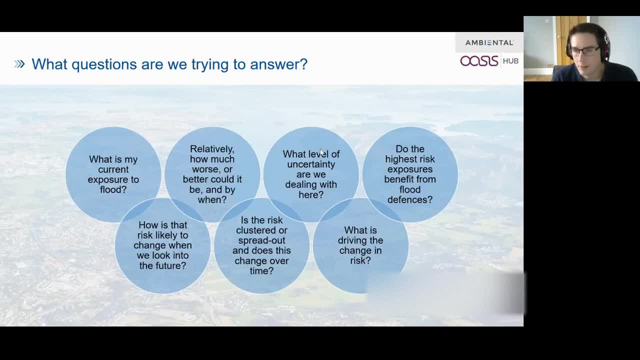 But more specifically, By when And what level of uncertainty are we dealing with? Do is that risk change spread out or clustered? Is it something that we could deal with as an organization by treating somehow a small section of assets, Or do we have to actually look? Is the risk spread right around the country and therefore it's more difficult? 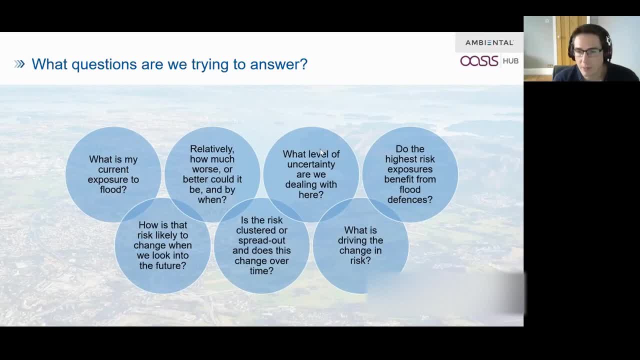 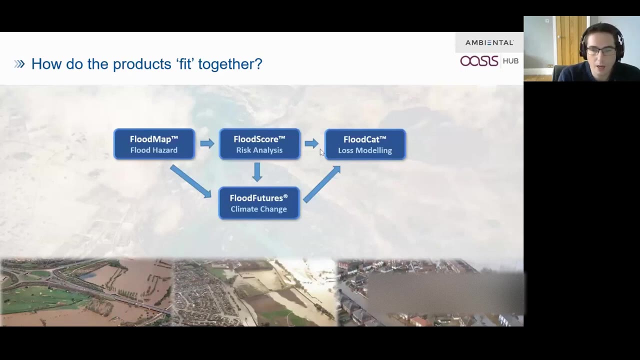 So answering some of these questions at this stage can be helpful for for making decisions on the medium, long and short term. OK, next, So very quick look at our products themselves. So I don't want to dwell on this slide of, just just a quick mention to say that everything that we build is is connected. 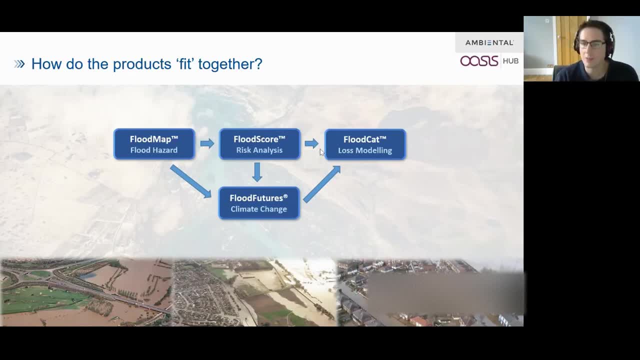 So the futures data sets are derived from the mapping and the scoring data sets, Or at least the same methodology to produce the mapping, So it all feeds through. So basically, a risk rating in one is the same as a risk rating in another. 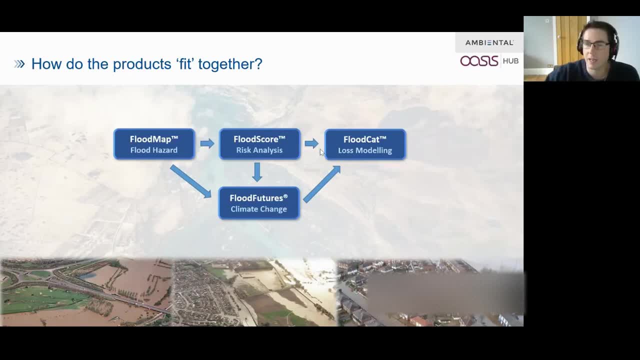 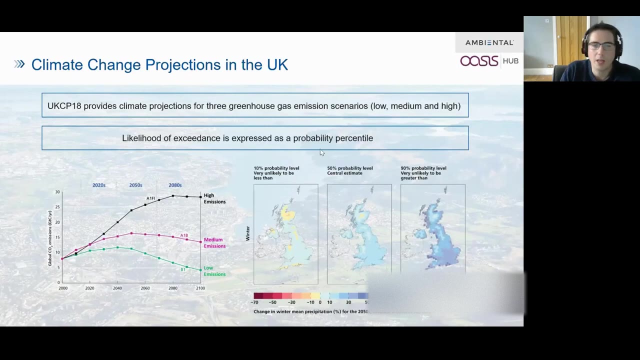 And that can obviously feed through into the CAP model as well. So everything is consistent and built upon one another. And the next Cool. So let's just think about the UK for a moment. So the UK Benefits from fantastic scientific basis in the UK CPO nine and UK CPA team programs, which have generated huge amounts of data and insight into into these challenges. 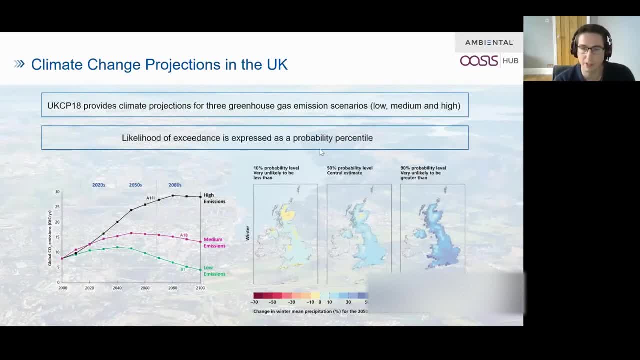 Far wider than just flood, of course, but we're interested in certain components And, given that we're dealing with uncertainties here, our approach to climate change modeling has been to provide three different pathways. And, given that we're dealing with uncertainties here, our approach to climate change modeling has been to provide three different pathways. 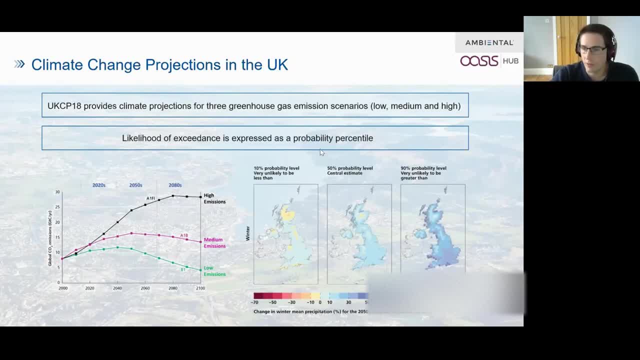 So broadly speaking we call these high, medium and low for simplicity. But these relate to RCPs, So our high emissions is tied to the eight point. five. medium to six Low has changed in the UK from from the used to be four and a half. 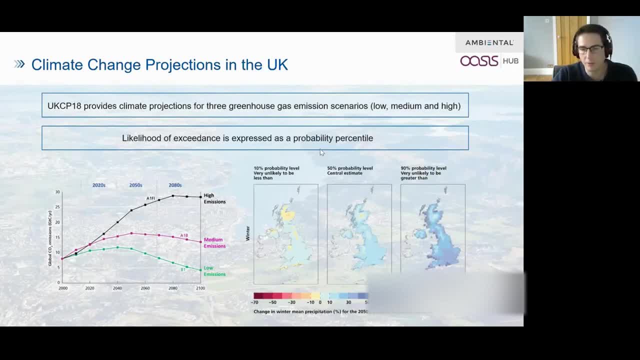 It's now two point six that we tied to. So it's a closer line to the Paris Agreement. And again, the point is, if we're making strategic decisions about something that we're uncertain about in the future, it's helpful to follow a single path and take that sort of more deterministic route. 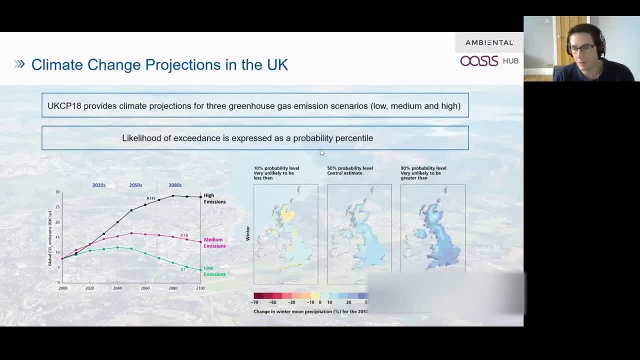 But we feel it's more helpful to follow that route, knowing what the upper and lower bounds might actually be. So, how bad could it be, even though it's unlikely? Well, how good could it be, although it's unlikely, And that that that's. that's a theme that we maintain throughout our products. 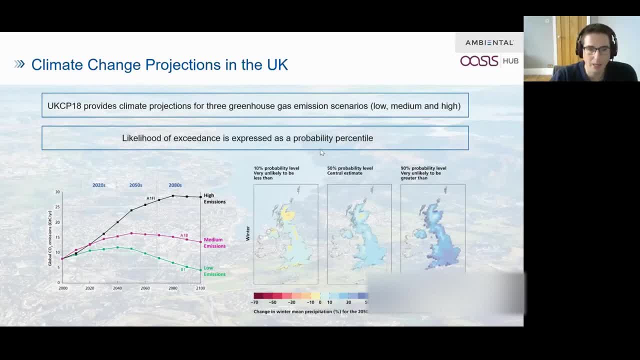 Now we don't have time to talk about that. We don't have time to talk about exactly how we get there. There's quite a few decisions to make along the way: how we treat the probabilistic outcomes from climate models, from UKCP. 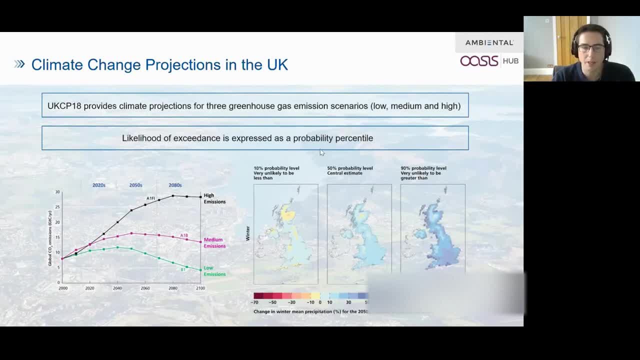 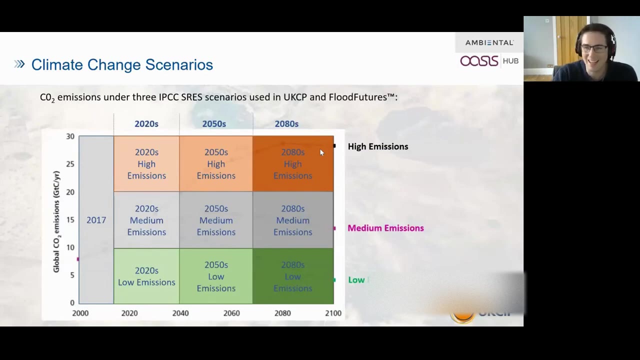 A little bit too technical for now. Very happy to talk it through with anybody at a later date. Essentially, we define these high, medium and low profiles and then project those into the future. Next, And this is just OK, Oh, that's supposed to come in nicely. 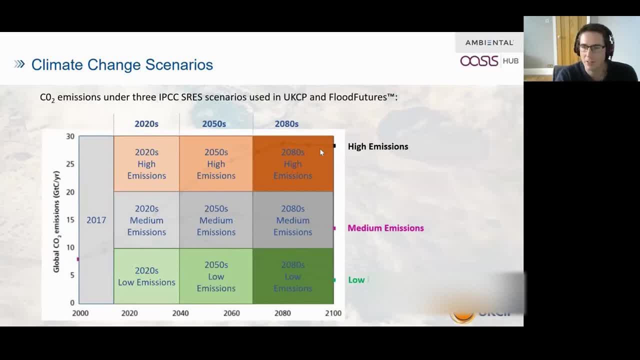 So this is just a zoom in This graph- that this is a matrix of essentially the nine future scenarios. So when we talk about climate models, we need to talk about points of time in the future. But this is even in itself difficult because you're not really talking about a single point of time in the future. 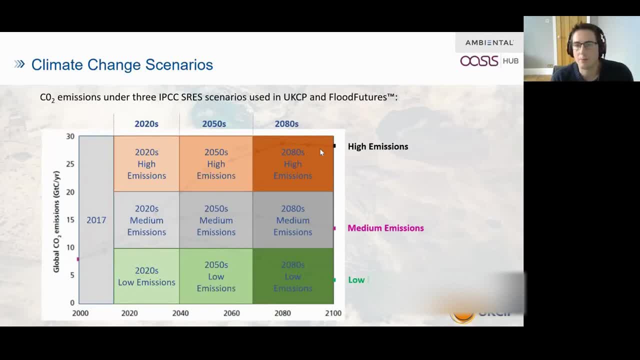 You're talking about a multi-decadal epoch, a chunk of time between now and the future, So, to put it another way, the 2020s. these climate models are simulating continually into the future, hour by hour, simulating our weather and other various systems. 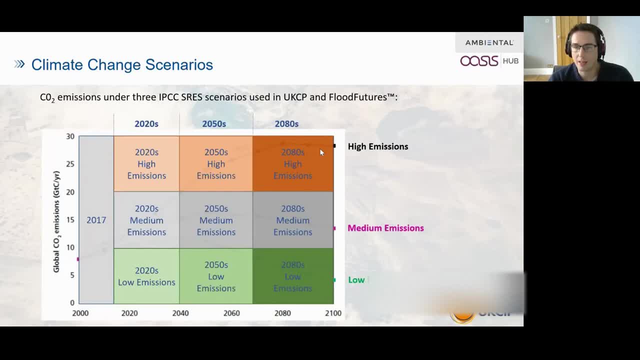 We basically need to average chunks of that to create what to us now appears closer to a point of time. So the 2020s is basically near term. It actually spans from the UK So from 2015 to 2039. So several decades of time. 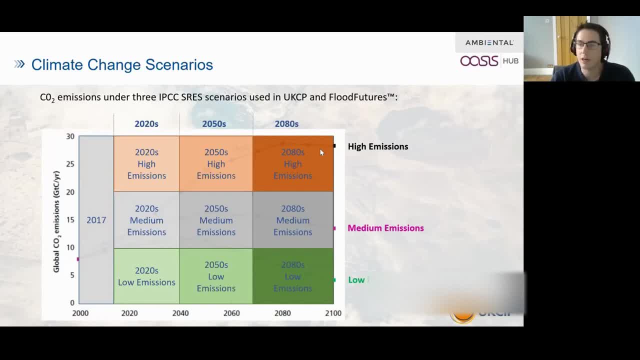 And that is averaged out a bit like we average out a flood gauge looking back for 30,, 40 years in order to try and explain what's going on now. So essentially, we deal with the same type of processes that we use now. 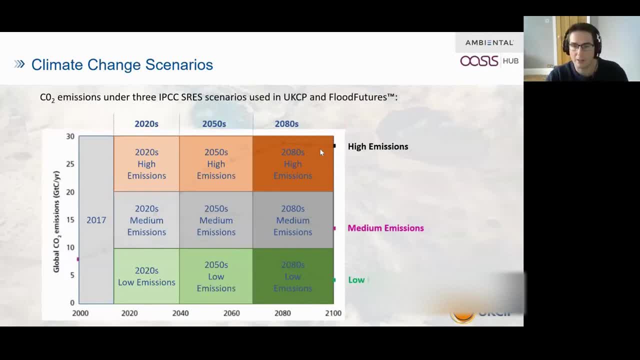 But we just imagine that we're in the future and that that has just happened. So 2020s, 2050s, 2080s, near-term, mid-term and long-term risk High, medium and low emissions. That gives a nice matrix of nine that you can follow through in time or follow through in terms of the emission profile and see how that impact can happen. 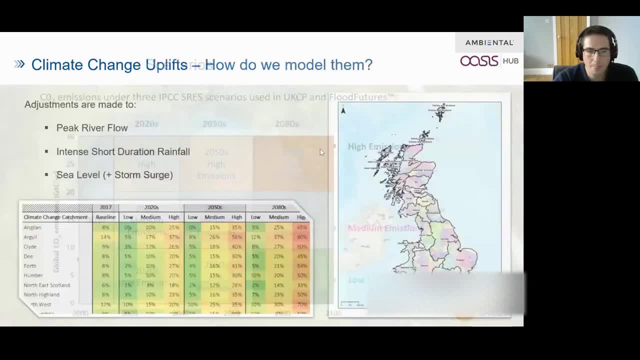 So next one, please, Rob. OK, So the big challenge that we have from climate change, Moving from climate data or climate model output to hydraulic flood map output- is we have to go via hydrology. So how does the climate model actually change the hydrology or the way that we view that hydrological model, in order to change what we then put into the hydraulic model? 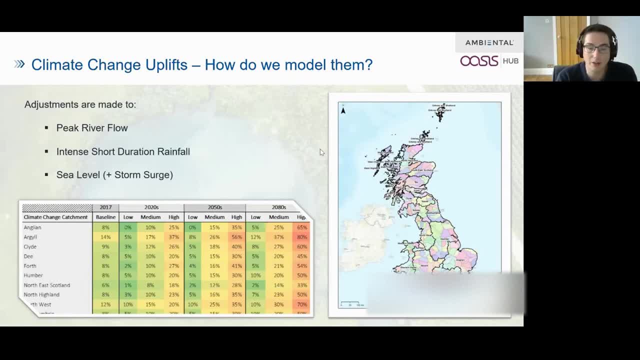 That's really difficult And there's a great deal of science that we've consulted in order to In order to get to this point, especially in the UK, where quite a lot of this science was done on the back of the UKCP data when that was first available in 2010.. 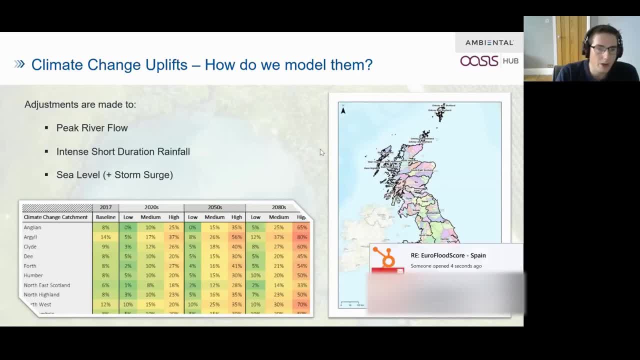 It came out after 2009.. So, essentially, what we're doing here is we're translating climate model outputs- which might be things like temperature changes or amounts of averages of rainfall, changes in power Or changes in patterns, into more specific things like short duration, intense rainfall or things like peak river flow. 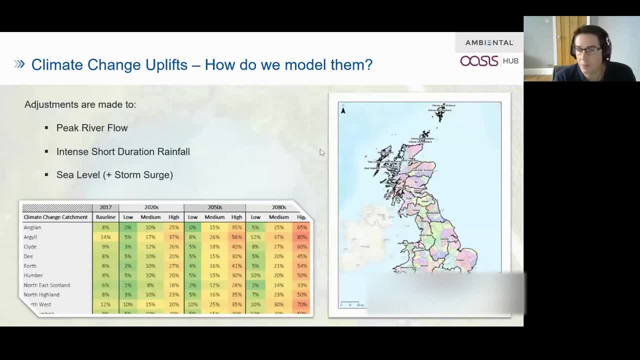 Most climate models will not touch peak river flow. That's a. that's a difficult concept to understand and is actually dependent on quite a few different factors that come out models. That is something that you can't just do. you know on just simplistically. 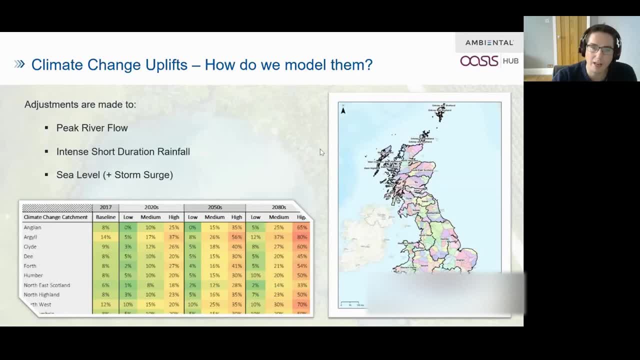 It's very difficult to. It's very difficult to actually understand how to translate one into the other. So that's where a lot of the work has gone in, with the, with the climate modeling projects that we've done in the UK and moving into Europe. 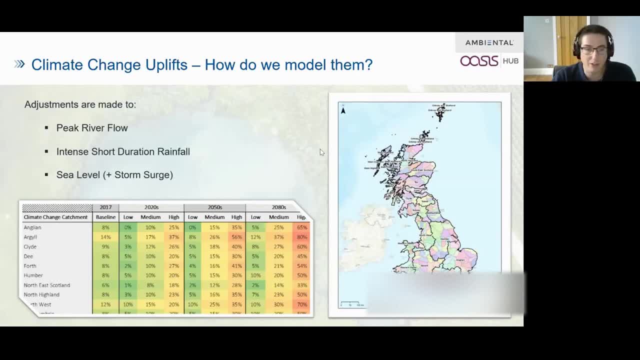 So there's lots of different ways of doing that, Some far more sophisticated than others. In the UK we've been very fortunate for using work that's come out of the Centre for Ecology and Hydrology, CEH. Some great work from the EA, NRW, SEPA, UQIR. 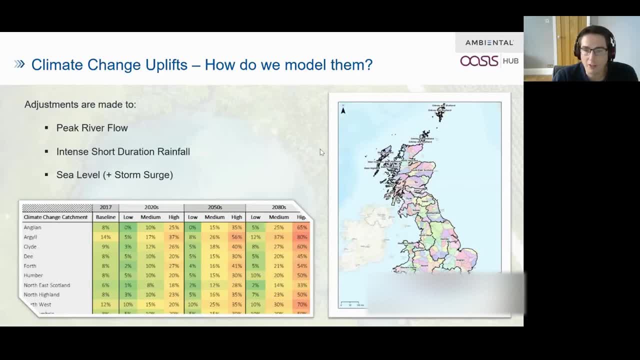 A lot of these organizations have produced science that enabled us to to then derive these, these products and these uplifts, as we call them, to our existing products. So this is just to put it into context. What we see on the screen now are some uplifts and changes to the fluvial models. 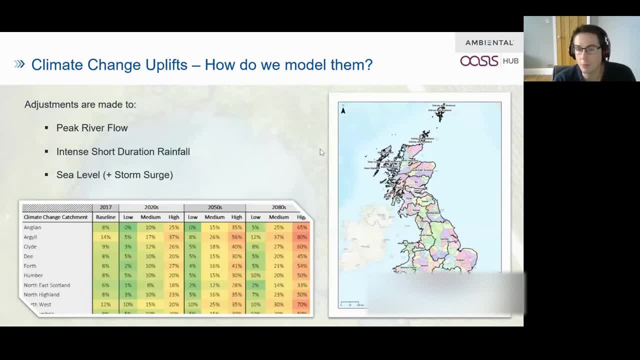 So this is the change in peak flow that you will. This is just a hundred year return period, The change of peak flow from now and into the future, Under the three different models, Under the three different scenarios. This is essentially what we need in order to then hydraulically model the output, which then can give us the impact and therefore the full risk equation at the other side. 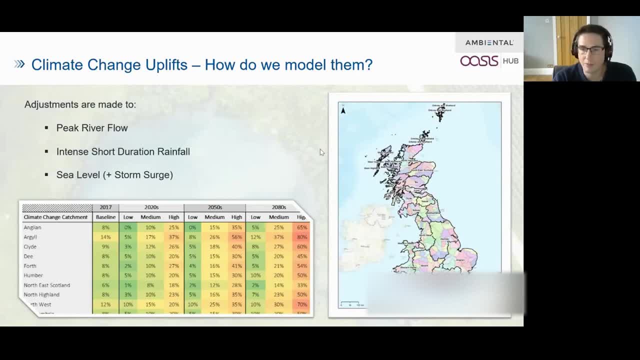 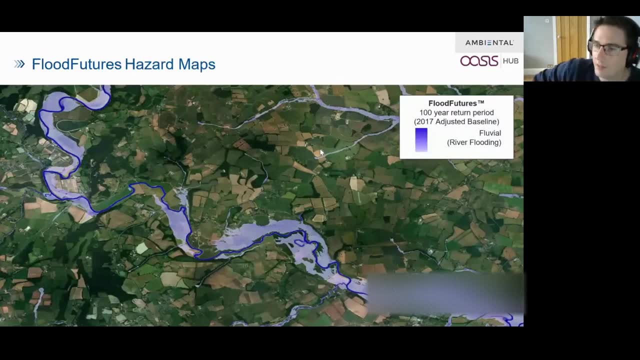 So that's where I'm leaving that. There's tons of information I've left out, of course, but essentially this is what we get. So this is again just looking at the hundred year. This is just a baseline for 2017.. 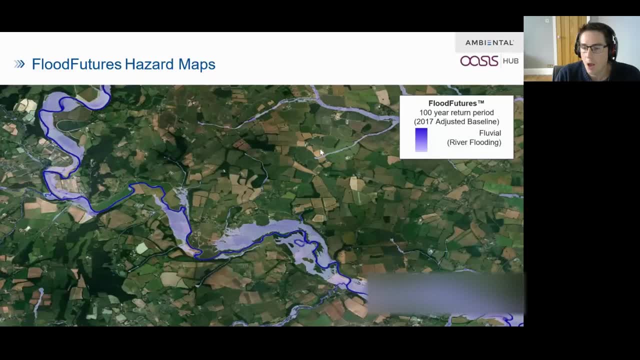 So essentially the now. Actually, Rob, can you just flick through these ones a little bit quicker? So this is moving into the 2020s High emissions profile. we're following now and then into the 2080s. You get the idea. 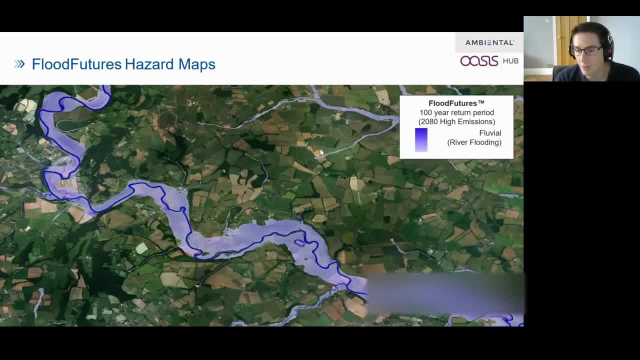 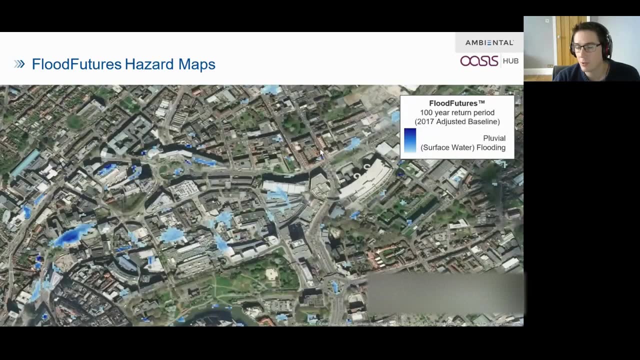 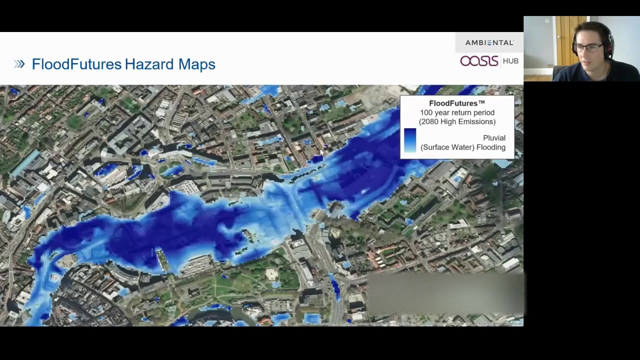 Essentially, flows increase for the same event as we go into the future and they increase more the higher the emissions. If you can keep going, Rob, This is the same for fluvial, A little bit more. So we're jumping into medium emissions 2050s here and then we'd make an enormous jump to 2080s high emissions. 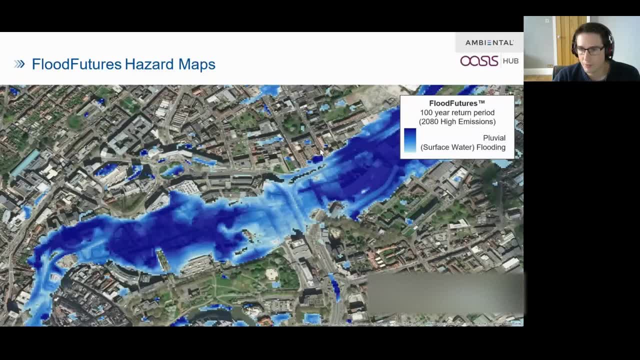 This is one of the most extraordinary patches of extreme risk we found. I think it's in Bristol, actually, where the drains were just overwhelmed by that extraordinary event in about 80, 90 years time. And these are the sort of things that you just wouldn't know without doing those kind of simulations. 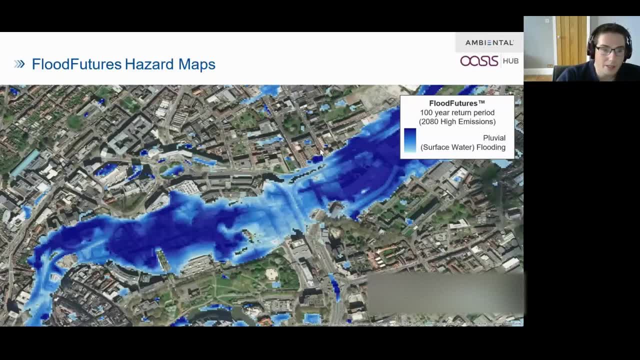 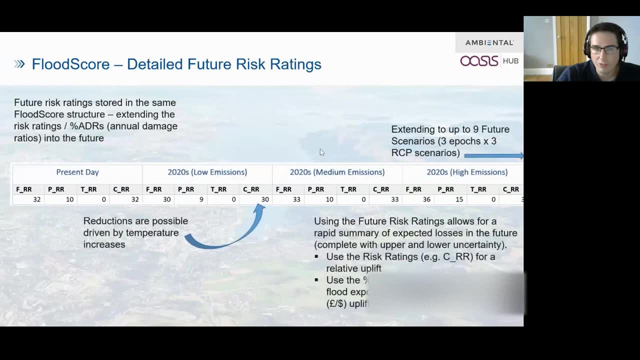 So that's, yeah, something that we're very keen to disseminate. Yeah, So the next one. So here's just a quick look at the Flood School products. These headings relate to fluvial, colluvial, tidal and combined. 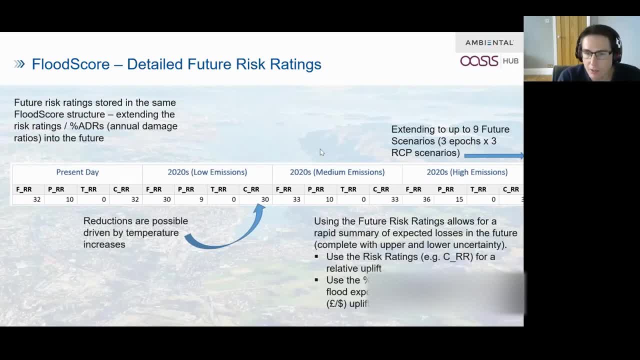 So F, P, T and R- Not going to dwell on this slide either because again, it's quite technical- But essentially this is how we derive our products. as Katie went through, For the future products we use the exact same format. 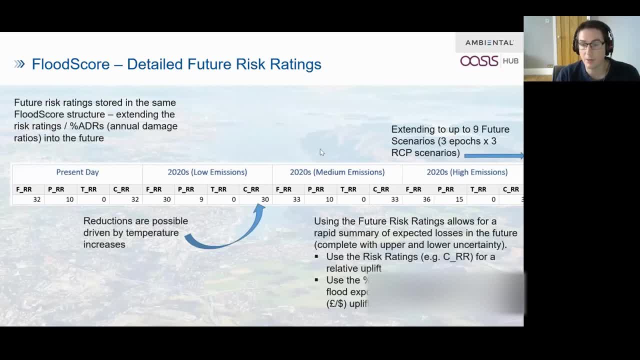 The techniques are quite comparable, relative, Of course. the risk might not actually go down, It might go up. Sorry, it might not go up, It might go down in the short term. That's what some of the modelling outputs are showing, depending on which emissions scenario you follow. 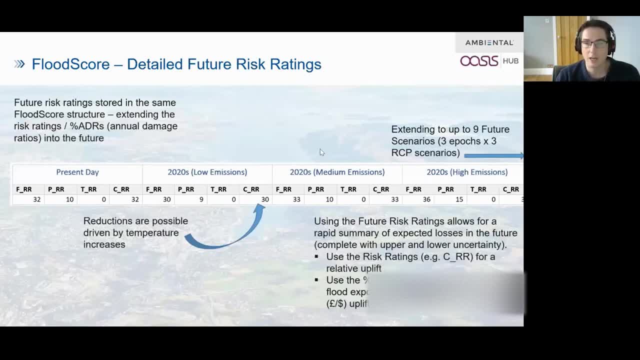 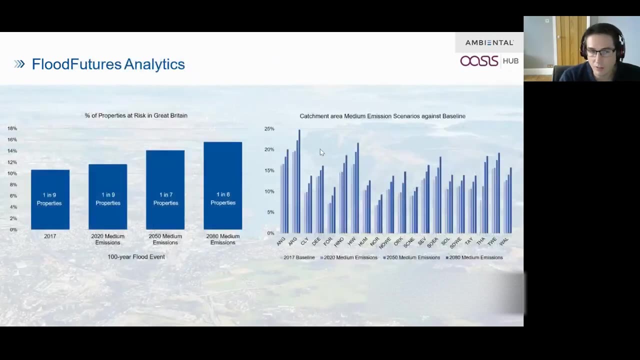 But essentially it just makes it easy to relate something in the future to now. And you can look at that with defences turned on or ignoring the presence of defences or whatever Cool Next slide. So yeah, this is just going to look at three more slides to go. 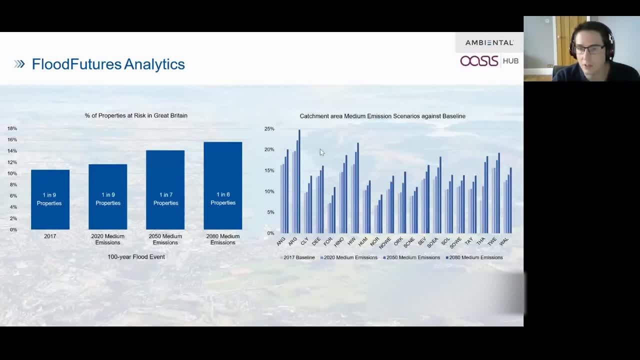 We're just going to look at three different ways that you can use the data. Spend about a minute on each. So this is just globally. globally, nationally, looking at the whole of Great Britain. The graph on the left is explaining the one again, one in a hundred year flood event level. 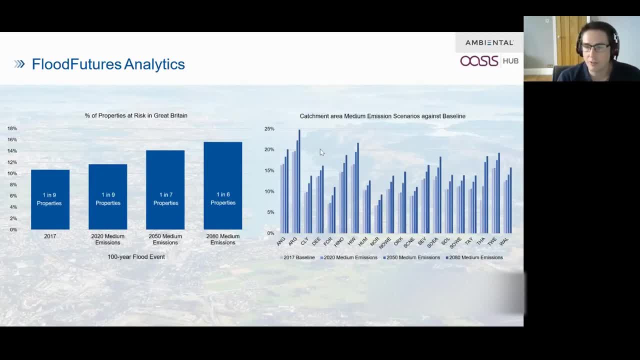 How many properties have some sort of potential impact. And that goes to the UK And that goes from one in nine today or a couple of years ago. It stays around one in nine as you go into the medium emissions profile. This is the 2020s, but it increases a bit. 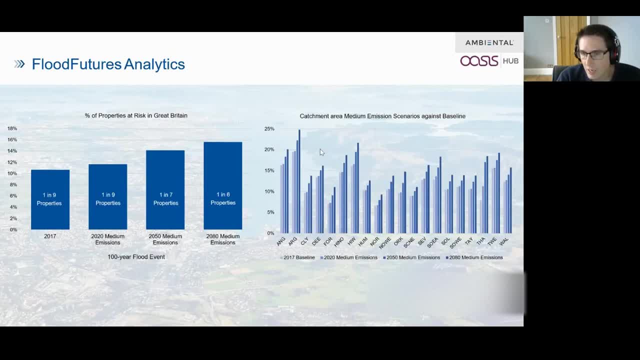 We get to about one in seven by the 2050s and then just about one in six by the 2080s, which is extraordinary really When you think about right now. it's fairly kind of the conventional wisdom, if you like. 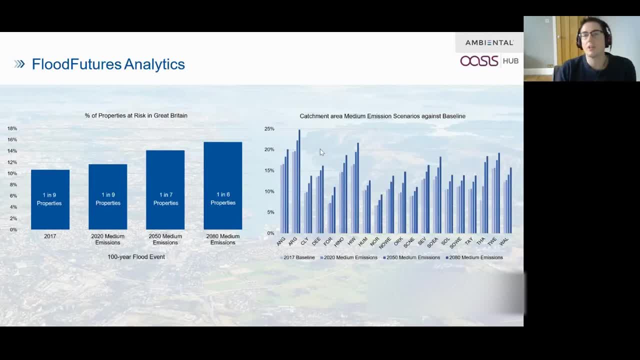 is that about one in six properties is at some form of risk in the UK. So that's the one in a thousand year, an order of magnitude less frequent, more severe event. And this data is suggesting that actually we might be moving to a position where actually that is the norm for the one in a hundred year event by the end of the century, which is quite startling. 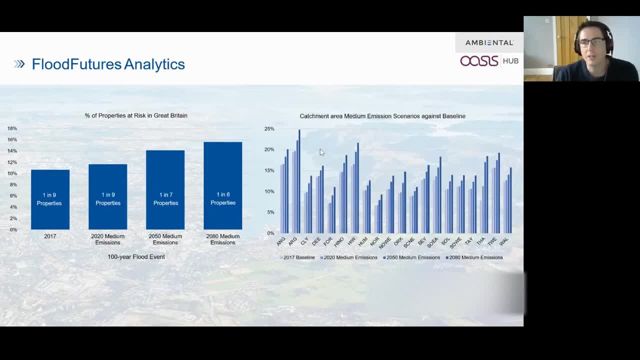 But actually if you look at that in more detail, what you find is much of that is just basically the surface water model and very shallow depths. So actually a better way of looking at that is looking at risk, So bringing damage into the equation. 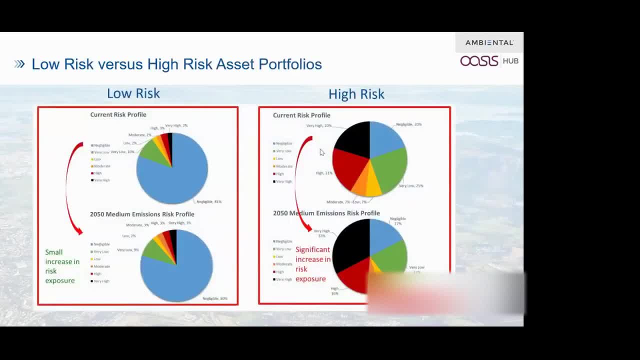 So, if you go to the next slide, this is how we tend to do it, for example, for insurance companies. So we can imagine these as two insurance company portfolios. So what we've done is aggregated the risk in this case. So we've got risk summarized into six bands rather than the 0 to 100.. 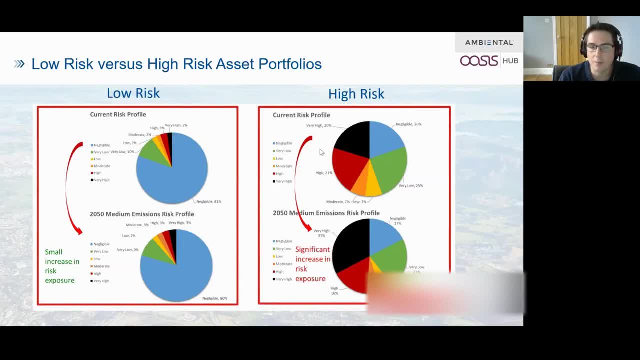 We just washed it into 0 to 5 by reclassifying it, And this could be an asset manager's portfolio, an insurance portfolio, whatever really- And what we're trying to do is say, all right, let's take right now, project it to 2050 under the medium emissions profile. 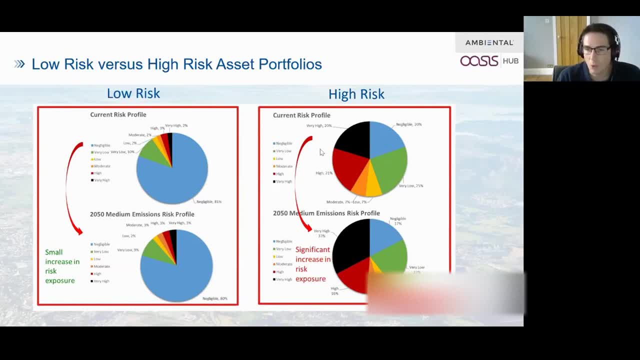 We're going to follow that one And let's just see what the, The shape of risk looks like as a pie chart in this case, at that point in time in the future or thereabouts. And what we found is quite interesting, In this case the 2050s lower risk starting point group. 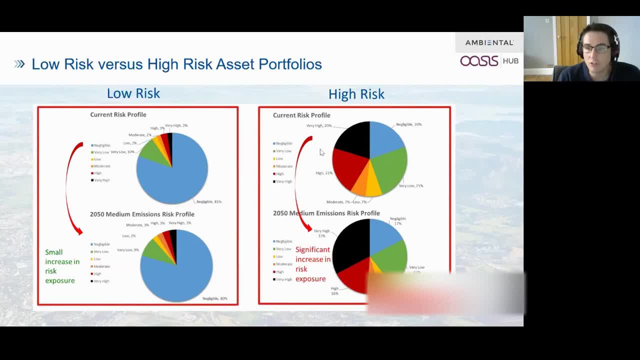 So in other words, the portfolio with relatively low risk now actually doesn't have that much more risk in the future. I mean really it's minimal. We've got only 1%. that's moved from negligible up to very low or something higher, which is, I mean, that's actually surprisingly low. 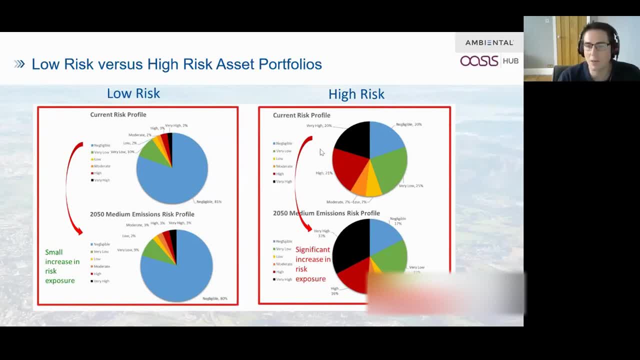 That's very fortunate. I think in this case it's probably you'd expect to be a little bit higher than that on average, But this is a randomness, of course, But really it's quite surprising that very little has changed on the aggregate. 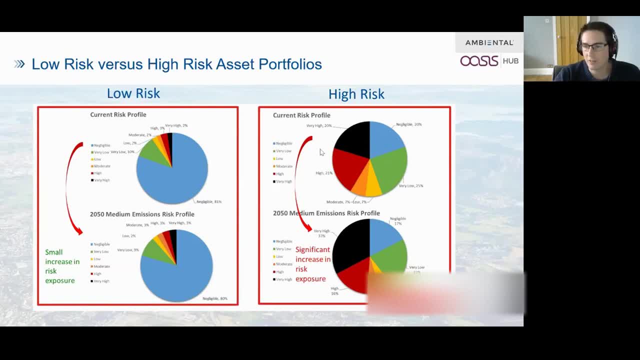 If we look at the high risk profile- and again of course we've selected for effect here- It won't be the same, It won't be the case every time, But this particular high risk profile really does show a significant increase in risk as you move forward. 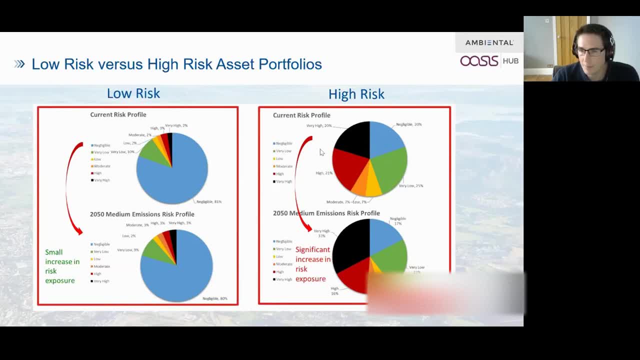 And that we found really quite, quite interesting. Particularly, this is properties moving up into the very high risk profile, And what that tells us is that the impacts of climate change with flood are just not linear, And that justifies- to my mind at least, it's worth going to this level of detail, to the property level, to look at this sort of thing. 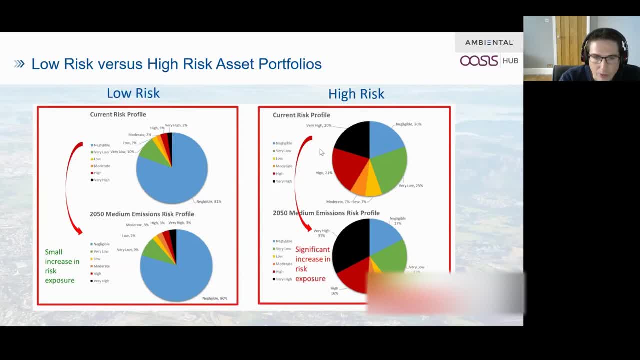 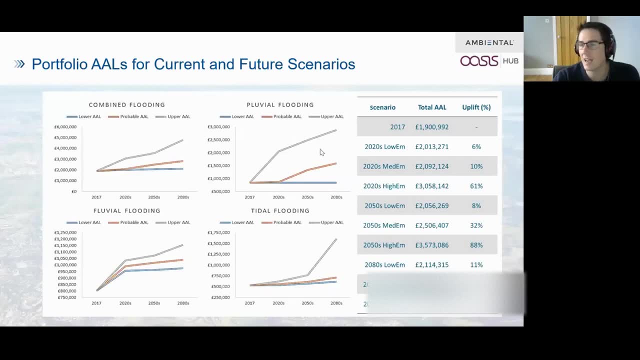 So, yeah, I think there's one final slide for the summary. We'll move on. This is just again another way of looking at a similar sort of thing. This is using average annual loss as the metric And everything ties together. whether you look at it, the risk ratings are derived from average annual loss. 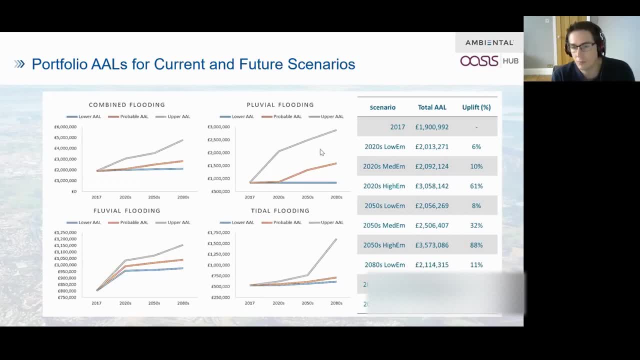 And this just shows all of the differences. This just shows all of the different future RCPs on the same graph, So you can kind of see which flood sources are more certain and which are less certain, Which in itself can give you more kind of richness of data to play with and get confidence one way or another in your mind. 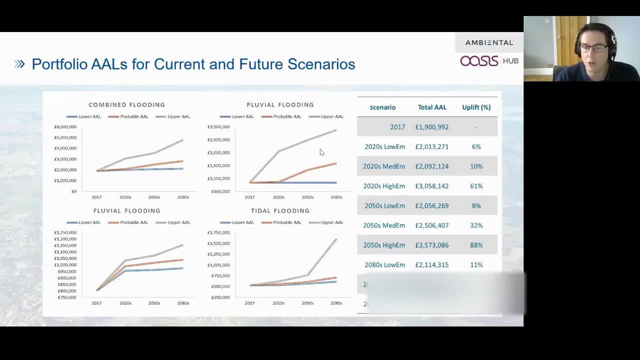 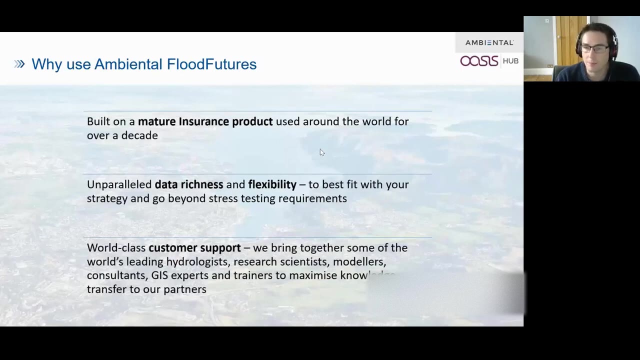 So ultimately, this is an uncertain thing And we're trying to just build as much knowledge around what might be as possible. So final slides And I'll leave it there. This is just a few benefits around why we've done it this way and why we've based it on our flood school insurance offering. 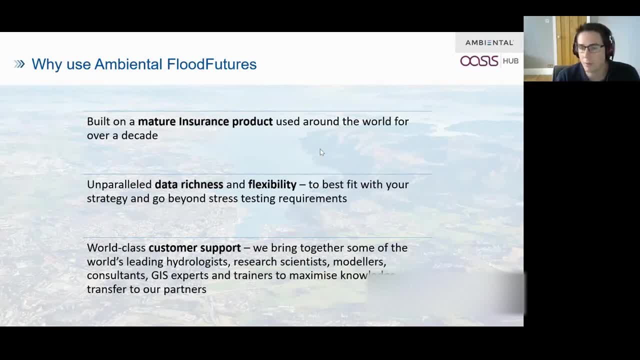 And really that's just to make it easy to work with, because not everyone wants to answer the same questions And not everyone wants to go to the nth degree of detail. But crucially, there is a massive replacement. There is a massive repository of data here that can be used to answer lots of different questions. 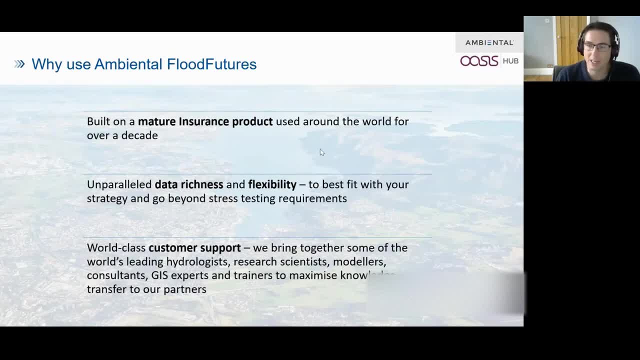 And the answers it will give can be very, very simple and very, very clear. And that's it. I'm going to leave it there. Okay, Thank you very much, David. That was a really excellent presentation and looking at really climate change flooding the future. 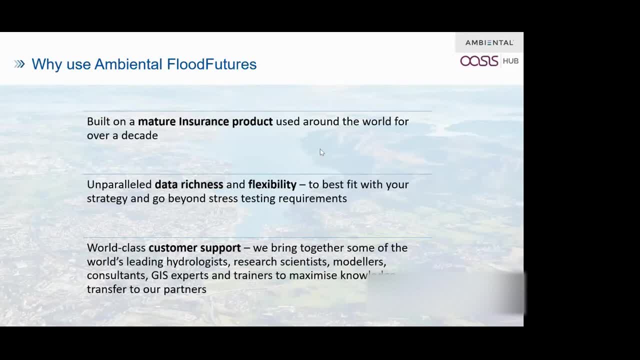 It's quite scary what it actually shows in the UK and Europe. Now I'm going to hand over to Rubini And she's going to go through the CAT modeling and focus mainly on the Australian models. Over to you, Rubini. Thank you, Rob. 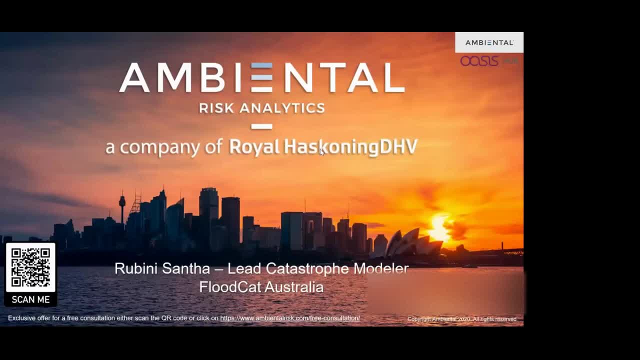 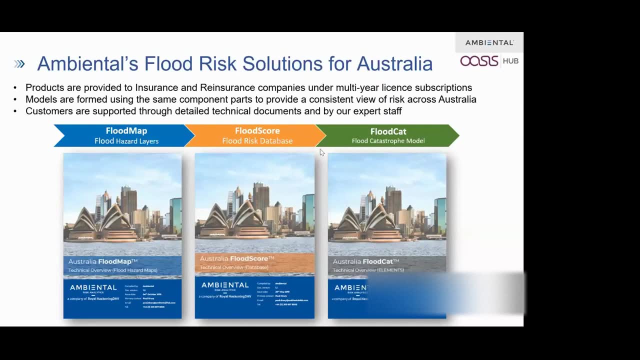 Thank you, Dave. Can we just switch on to the next slide please? Yeah, So my colleagues Katie and Dave spoke about the production of flood map and flood futures and things and its key features. So in the next few slides I will be talking about how flood score, especially the property level flood score, risk rating, is used in the development of flood CAT. 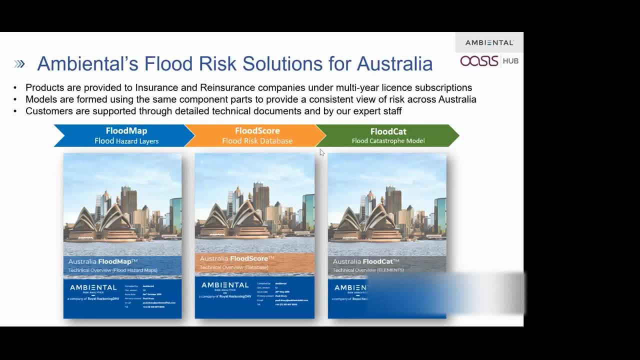 And, most importantly, how the changes in the production of the flood score, that is, the risk rating database, impacts the flood CAT results. So here's a slide which tells us like how the flood score and the flood map ties into the development of flood CAT. 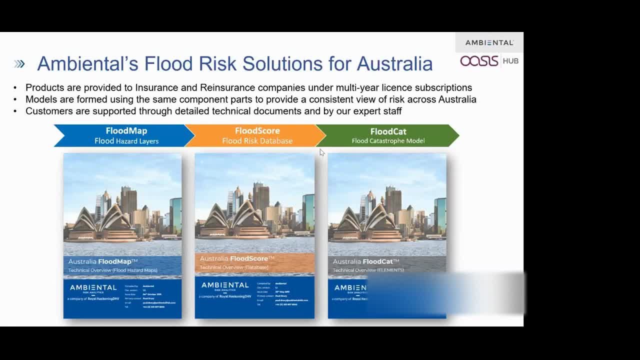 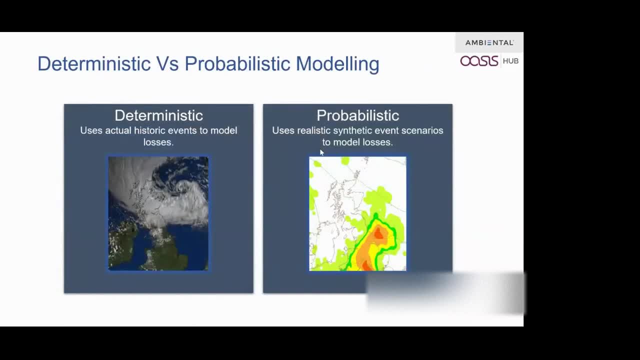 This is just an introductory slide. Can we move on to the next slide please? Right Before we head on to the development of flood CAT, I would just like to touch base about the deterministic and probabilistic modeling. So most of you as you know, a deterministic model is meant to yield a single solution describing the outcome of an experiment, given appropriate inputs. 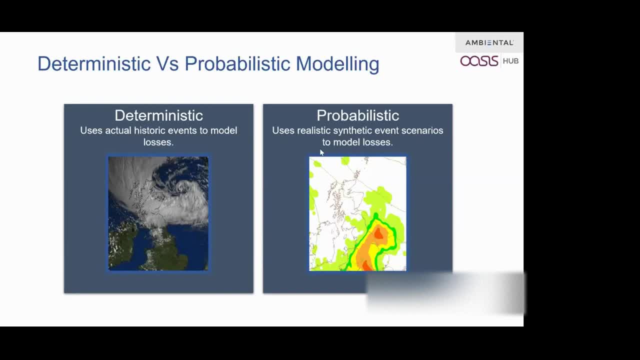 Whereas a probabilistic model is instead meant to give a distribution of possible outcomes, That is, it describes all outcomes and gives some measures of how likely each event is likely to occur. So, in a nutshell, a deterministic model does not include randomness at all. 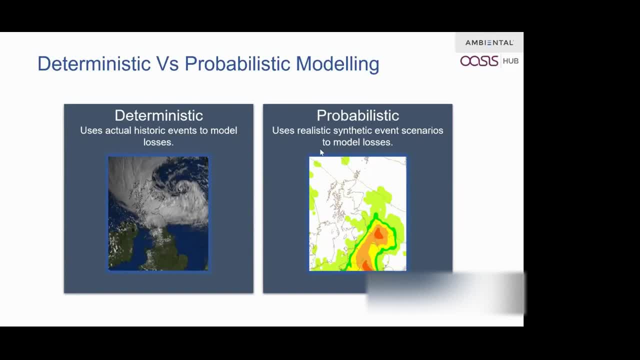 Every time we run the model, we get the same exact results with the same initial conditions, But when a probabilistic one, we will give different results each time we run with the same initial conditions. So these are the basics of how we are going to deal with the further slides going forward. 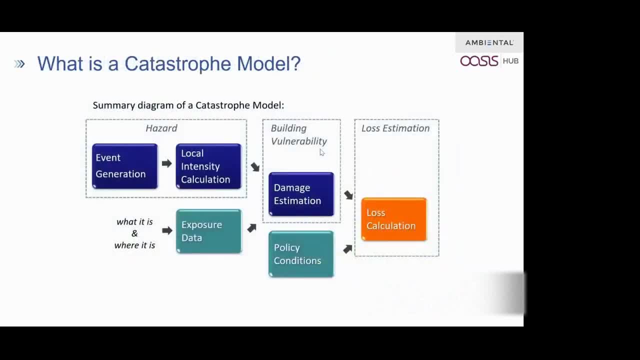 Next slide, please Right. So here are the principal components of CAT model And before that, what is a CAT model? So the commonly accepted definition for a CAT model is: it is a computerized simulations that use scientifically derived physical models to estimate where a catastrophe event will occur and how severe they will be and how much damage they will cause to properties. 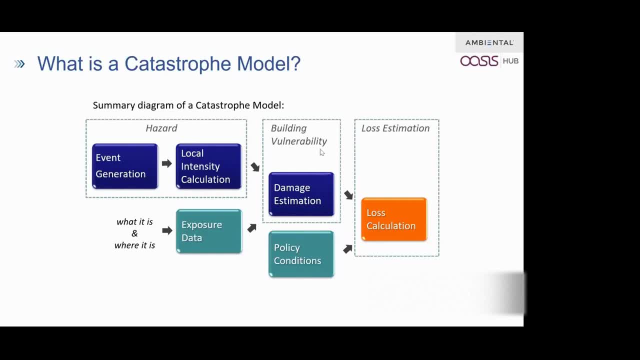 And most importantly, as we all care about, what financial consequences will it produce to the stakeholders. So this is the most accepted and simplest definition for a CAT model And here are the components which actually go into a CAT model. The first main component is a hazard model. 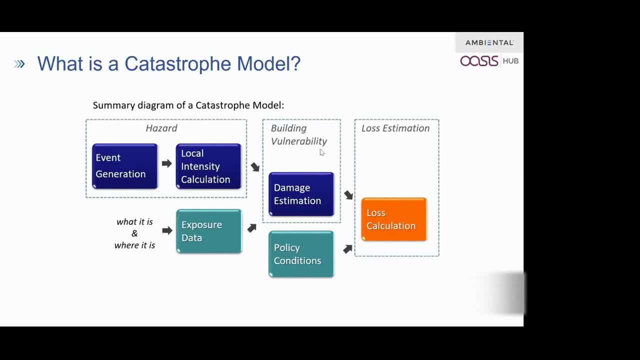 The second one is the vulnerability And the third one is the financial module. So there are two sub-components in our hazard one, which is the event module, and the local intensity calculation. I will quickly touch base on all these simple components before we get into the actual discussion. 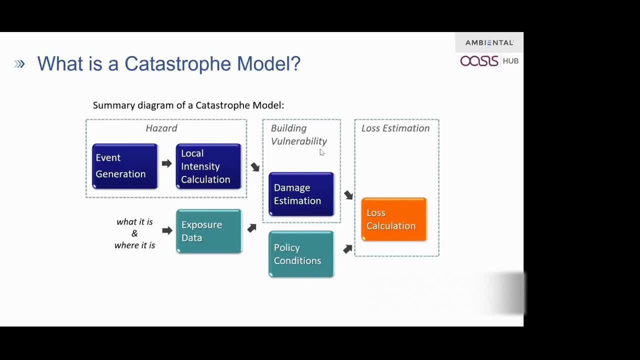 So in case of event module, it is just a database of stochastic events, So it is usually created using the past events and also stochastically simulated events that may not have occurred in the past. So, just like it includes the flood, future components, what Dave just spoke. 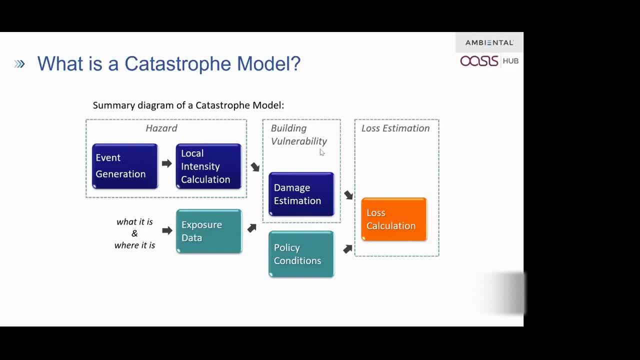 And for each event in the set, its physical parameters, such as location and annual probability, are defined. So the next one is the crucial thing, which is the location intensity calculation where our hazard map components, which my colleague Katie spoke about. So in this case, where the location and local intensity calculation comes, for each simulated event, the intensity of the hazard is calculated. 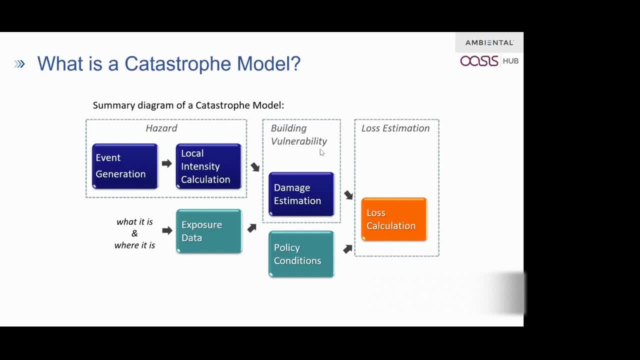 It comes from the local intensity calculation And the hazard is calculated at each affected site. So, in short, I would define this as hazard as a consequence of the event that caused the damage And the next part for the hazard component itself. I mean, it's not technically inside the hazard component, but it is directly linked to the hazard one, which is the exposure data. 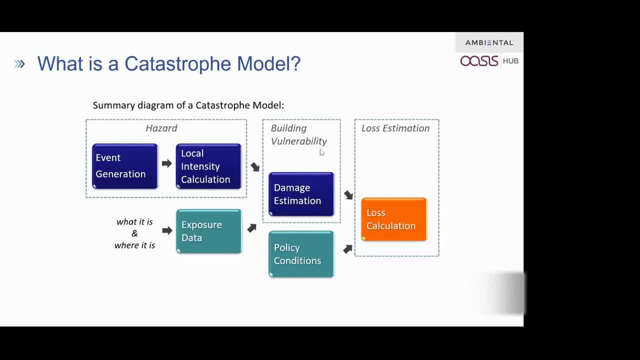 So exposure data is the information about the property, which includes physical characteristics, replacement value and so on. So in this case, for this case study, it would be Australia And there we use the data. The data is represented as GNAS, which is the geocoded national address file, which has the latitude and longitude information and all other information that I mentioned previously. 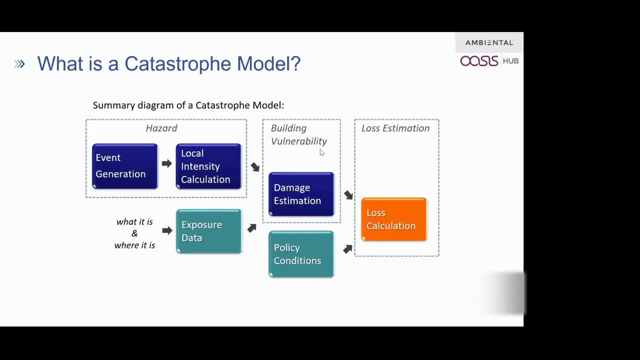 These two components feed into another module, which is the vulnerability one. So where the damage estimation happens, So the damage estimation, where the physical damage is calculated for each affected exposure. Going forward in case of the damage estimation component, where the vulnerability is the key, 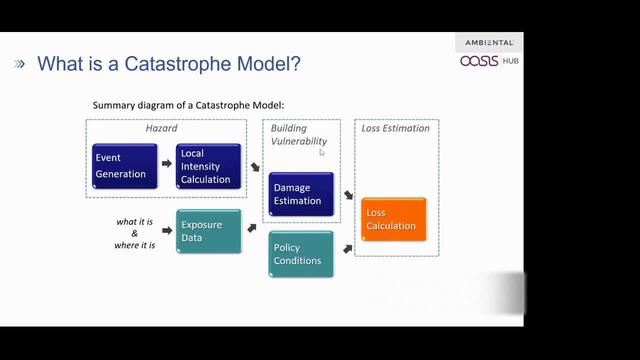 where the vulnerability is the key. the vulnerability function is. it completely varies for each building. for instance, it will change in the basics of the various building characteristics, such as construction type or age of the building, or the height and occupancy type, and so on. we will discuss about how this vulnerability actually influences the 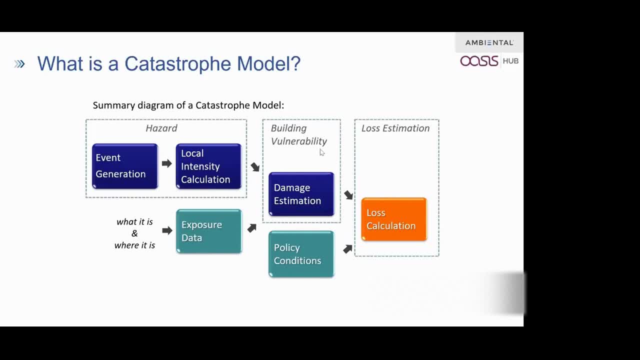 cat model results and maybe after four or five slides from now. last but not the least, all these things tie into the, the expected result, which is the loss estimate, loss estimation. so in the loss estimation, this is a stage which converts the damage ratio from the vulnerability module. 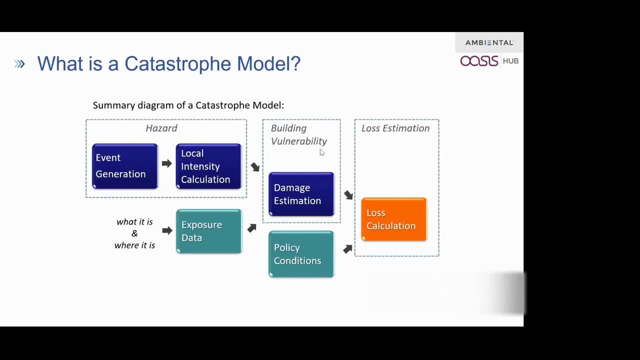 into financial loss. the damage ratio function for the specific event is multiplied with the building replacement value, which is which is usually known from the engineering, engineering codes, and which gives us two different components, two different outcomes, which are the als and ep curves. we will discuss about what, the what these outcomes. 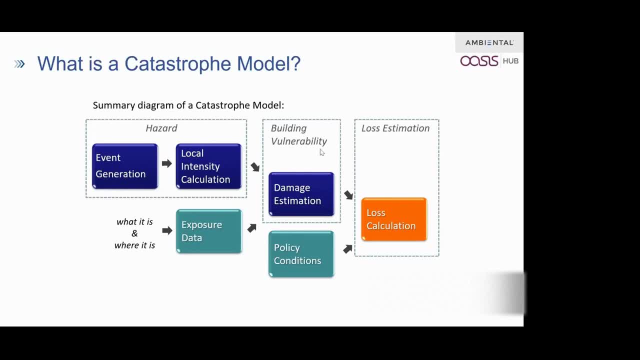 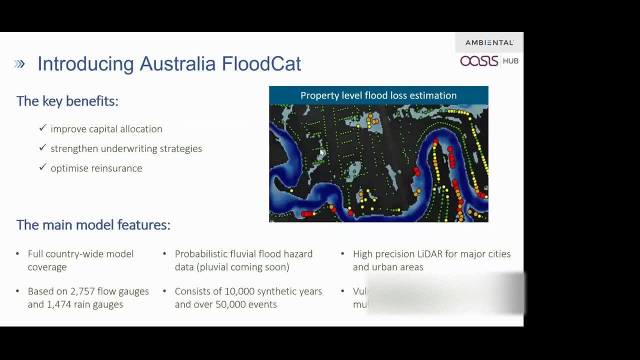 are through the end of the slide deck. next slide, please right? so we talked about what is a cat model and what are the components which go into building a cat model, although we haven't discussed what are the outcomes of the cat model, which we will keep. we will keep the placeholder now. so what? 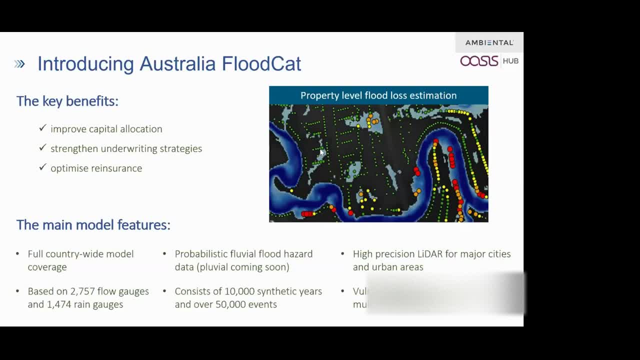 is ambiental. australia flood cat offers. so i've mentioned about the key benefits here and mainly i want to focus on the model, main model features. so in the previous slide we did see about the importance of hazard and the property and exposure, because these two are the main ingredients which is going to which. 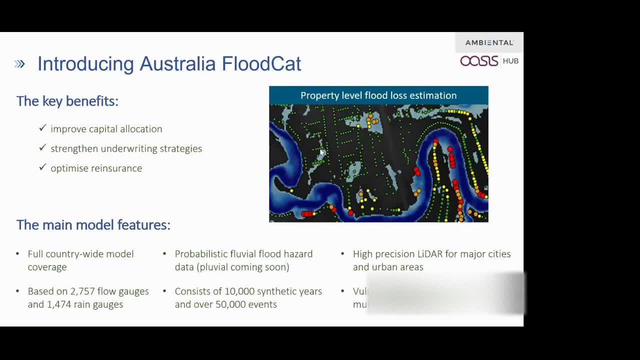 is going to impact the results for the loss of financial loss estimation. so in our thing in case of hazard, so we have- katie has covered all these things, but i just want to reiterate this again- so we have a full country-wide model for australia and for the hazard production. it is based on two. 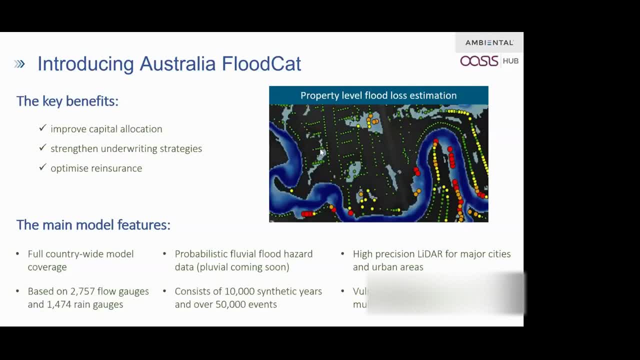 two thousand and odd flow gauges and thousand and odd rain gauges and for the synthetic database for when we are protecting the event set which are stochastic. here we have about ten thousand synthetic years and over fifty thousand events and coming to the exposure data, we have high precision light of a major cities in urban. 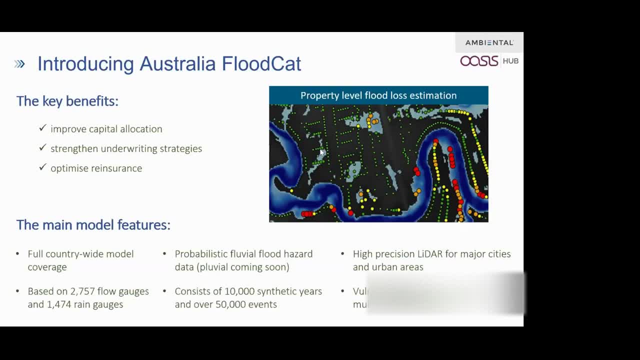 areas. why is this important? why am i reiterating on having high precision lidar for major cities? we will answer this by end of the slide deck. that's going to be the major discussion for this piece. and, last but not the least, the vulnerability data representing multiple. 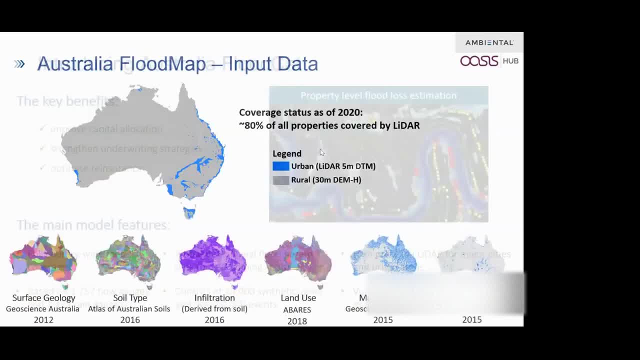 building types. thank you, no, you were right, you were spot on time. so here is what the input data for the hazard and for the exposure data goes into. so we have the coverage status as of 2020. we have 80 percentage of all the properties is covered by. 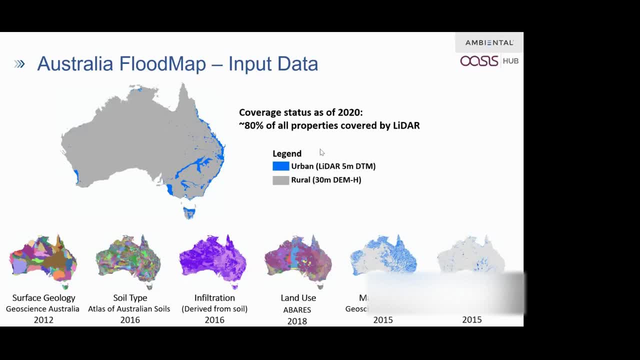 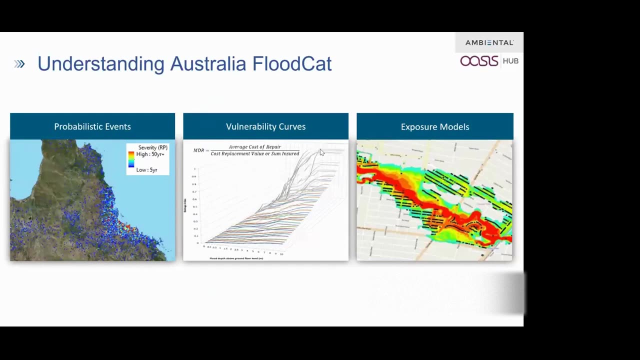 lidar. the blue color represents the urban one, urban model, and the gray one goes for the rural one. so this is just a pictorial representation of what we have in there. next slide, please. right? so we talked about the cat model is, so it was more technical. and then we talked about how. 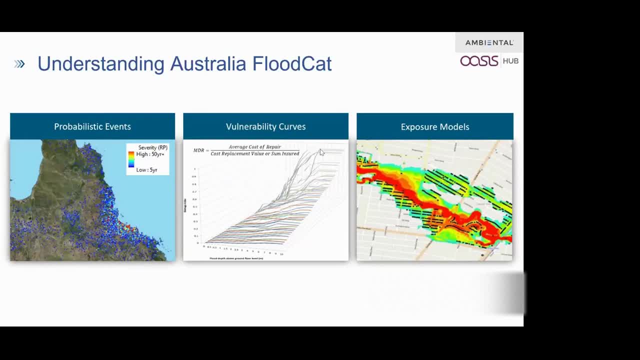 australia cat model. uh, flat cat looks um, ambient and split cat looks like. but this is more of um, there's more of um. so i just wanted to give you a pictorial representation of how an event looks like because for the non-cat modelers it, i just wanted to give you like a feel of how an event looks. so 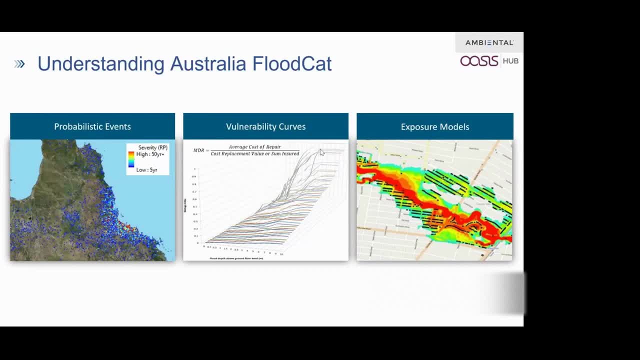 to your left. what you have is a probabilistic event, so it is um, so it is represented in blue. whatever is represented in blue, it is um, the lower region period, and whatever is in red is all high written period. so, in the view of time, i would just like to go to the next slide. this is all just a pictorial. 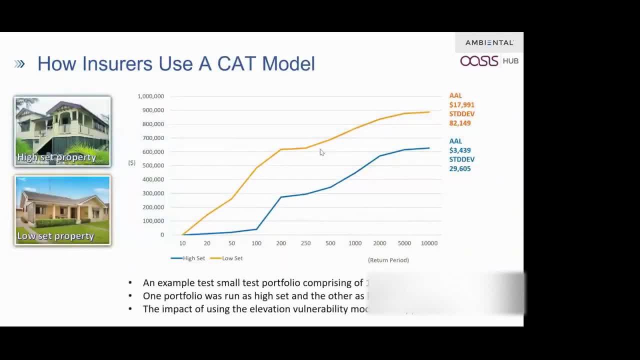 representation of what i spoke, so we're not missing anything. uh, now how do insurers actually use the cat model? so this is a classic example. so what i did was we ran a portfolio which has about like 10 properties, and one portfolio has a high set of what you see on your left. 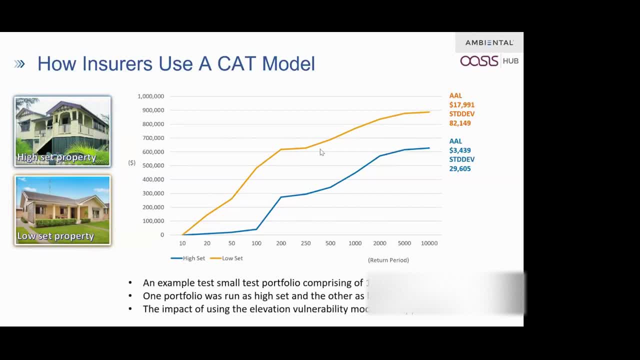 the topmost image and another one with the low set. so, uh, a logic here is is met, because when a same happens, the low set property is likely to suffer more loss compared to the um high set property. so this is a classic example which tells why it is very important to have the um, the primary modifier. 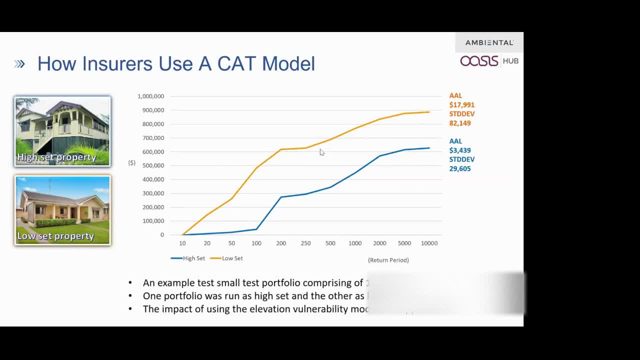 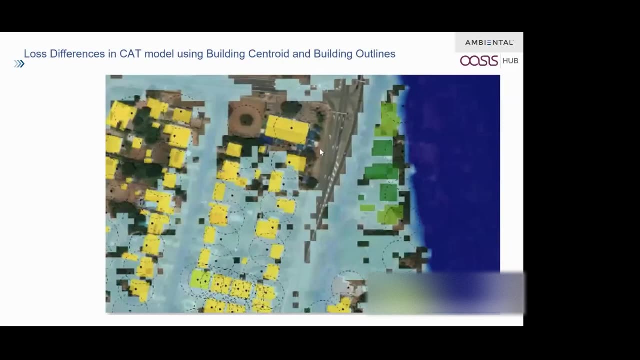 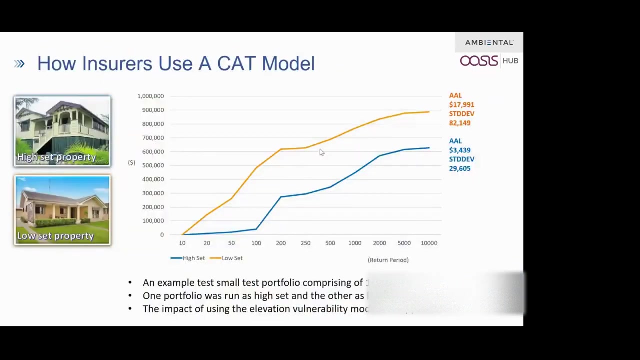 such as like elevation into your exposure database. so the the more detail your exposure database is, the more the your results are. more is more uh, reliable. uh, next slide, please right um, i'm i actually missed to say something about in the uh previous slide, about the outcomes of which i promised. the outcomes of the cat model are usually, yeah, sorry, so um, the outcomes. 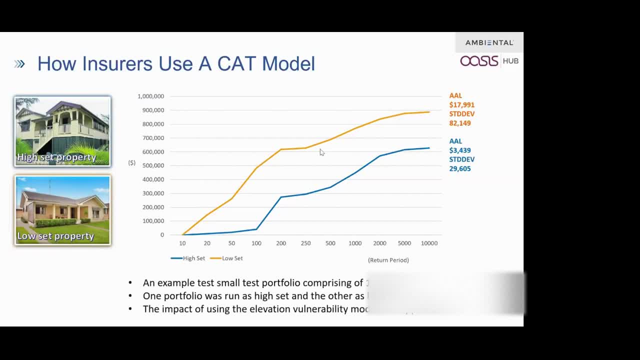 of a cat model are usually two things. one is the ep curves, which um the practitioners usually call it as exceedance probability. it is a probability exceeding a specified loss threshold, and what you see here is this metric, which is commonly accepted, which is the average annual loss. this is an 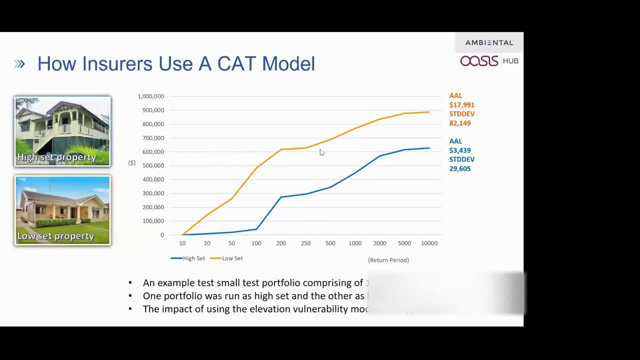 expected amount of loss from all the events in a given year. so we have 10 000 synthetic events and about 50 000 uh 10 000 event years and 50 000 events. so when we calculate the amount of loss from all these events in a year, you get the 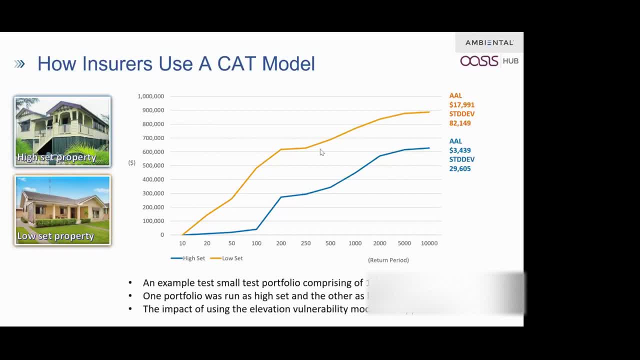 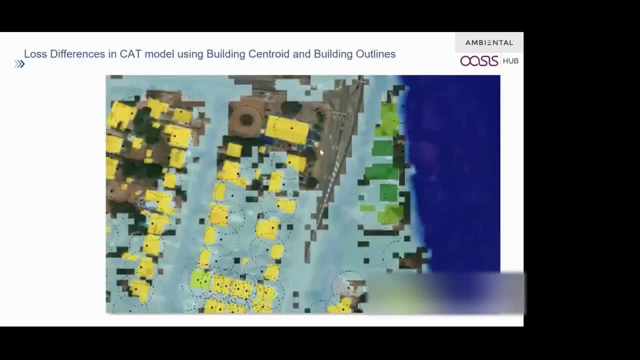 al. so this is a metric which is commonly used to um to uh, commonly used for a cat model. next slide, please. so, katie and dave and we all, we all talked about how important it is to have the property level detail models in our um, in our products. so this is a classic example where i want to just 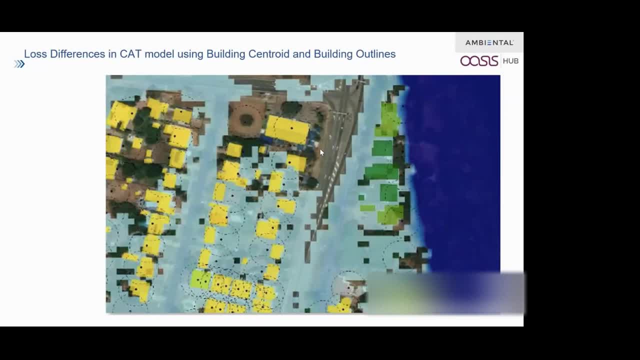 this is the picture where i just wanted to focus for a minute, which says: like the circle with the dot shows the exposure data set, which is a building centroid and its 15 meter buffer is shown with the dotted circle the risks. so so you here in this. 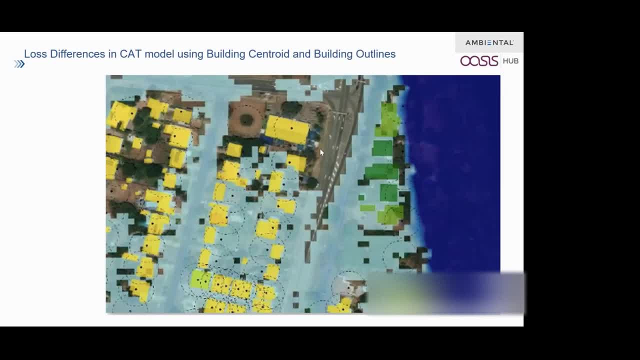 image we have like actually two databases. the one database is one with the dot and a circle, another one is a polygon. so the risk score is based on the buffer shown in a dotted line. for database one, or we can call it as flood score one and flip, for the flood score two, was derived on the polygons. 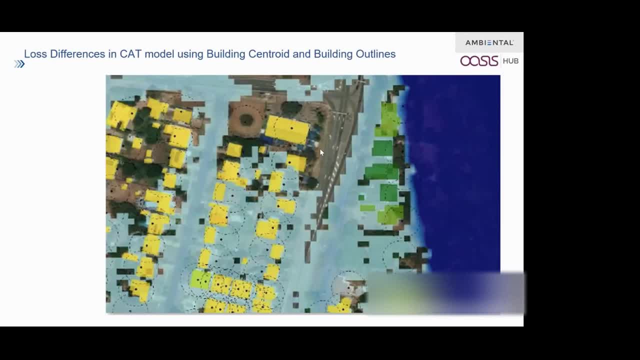 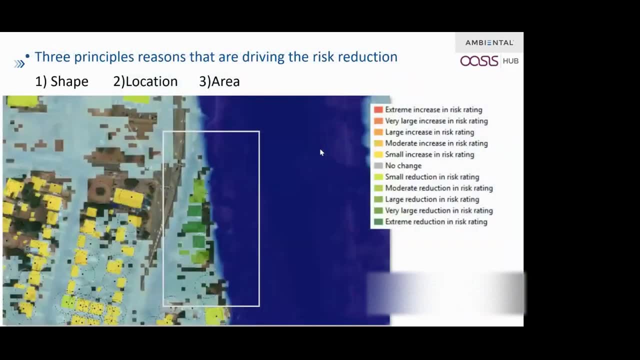 you see, which is the actual building outline, which is the actual building outline which represents the true shape of the building. so we will, we compare these two data sets and up next, like this, which has the results actually. so, when the risk scores were compared between these two data sets and the delta was plotted, 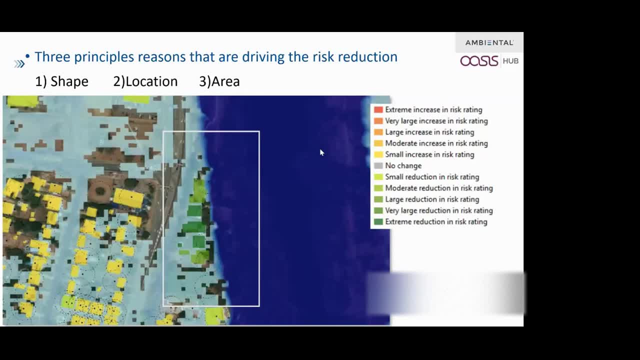 and color coded, we noticed some interesting results. so let us just focus on the box area. here there is moderate to very large reduction in the risk rating when we use the building outline. so the green one, the light green into dark green, it showed like there is moderate to very. 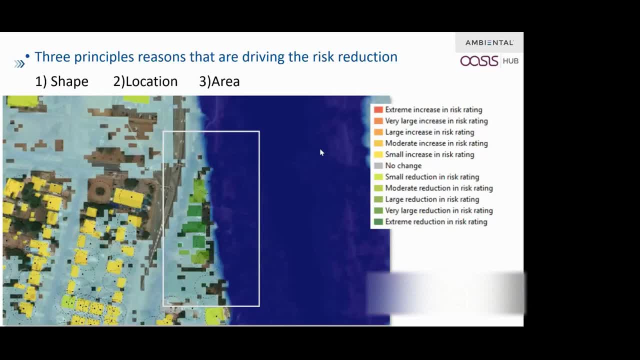 large reduction in the risk rating. so what is causing these three? um, what is causing these three? this, this reduction, this, this, this, this delta? so the three principal reasons were location, shape and area. so what is why is location deriving this change in urban areas? there is good correlation. 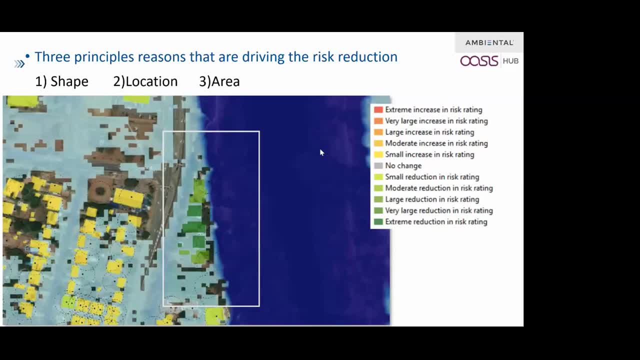 between standard uh address point and the building footprint. so we don't really want to worry too much about that. but in case of the rural one the points can be quite far from the building location. so if the point is that not actually in the building location, that means it is not truly. 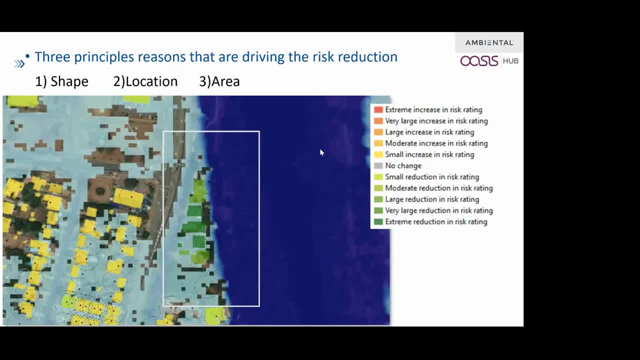 representing the risk in that given area. secondly, when even in even understand, even in the urban area, if the gnavs points are rightly placed within the building- they're often placed close to an edge- we will actually see that, um, how that actually influences the risk rating. the next slide, but 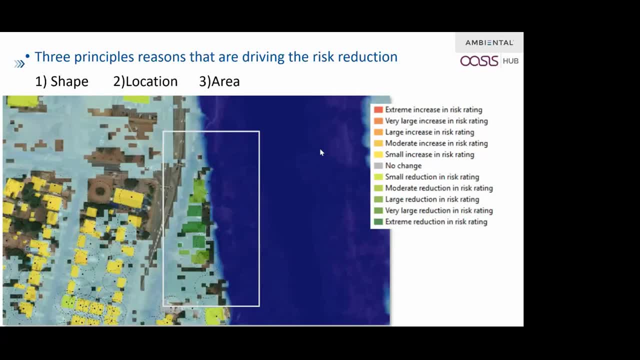 not right away. um, because in the waterfront property structures are located in the most elevated position within the land parcel, which are well captured by the building outlines but not by the central central points. so i want to skip through the shape and area, because the most important thing is the. 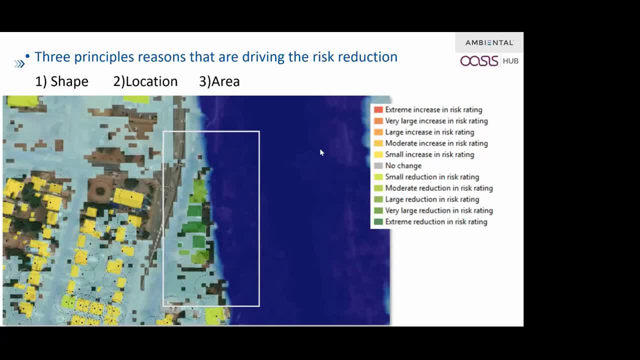 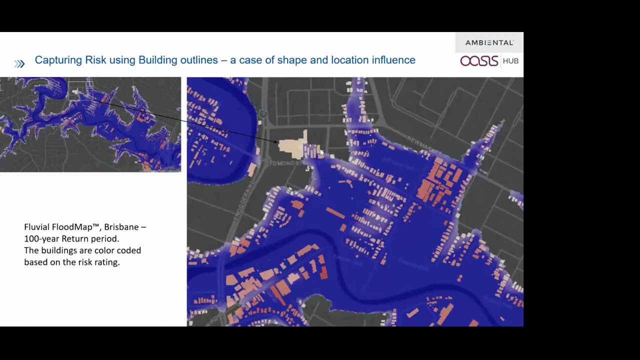 location. so that's how location actually influences your risk rating, which is why we reiterate on having property level database for your risk score. next slide, please. so this is a classic example. um, if you look at this one, this um building polygon, if your centroid was placed towards the left, it. 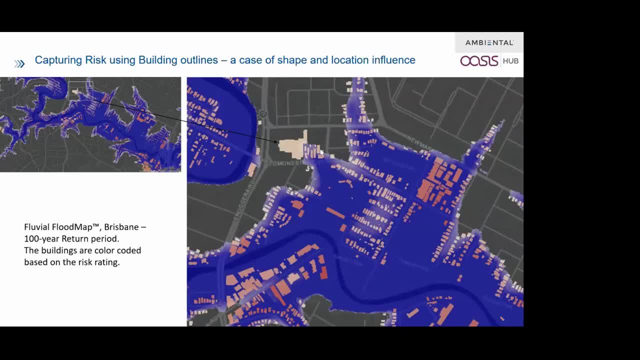 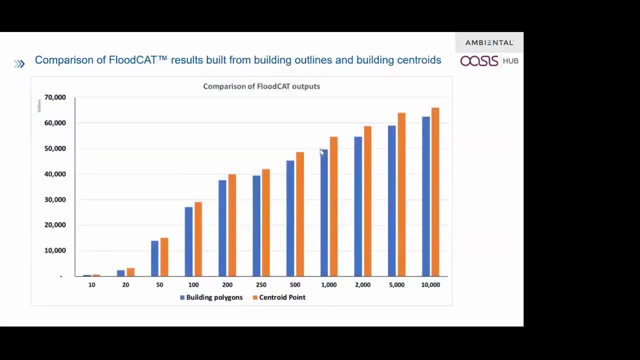 would definitely be missing the actual risk score. so this is the reason why we advocate having a building outline, because this captures the right score. right risk from the building, uh, from the flip plane. next slide, please. all right, so this is the case. so we compared about 1.5 million records. 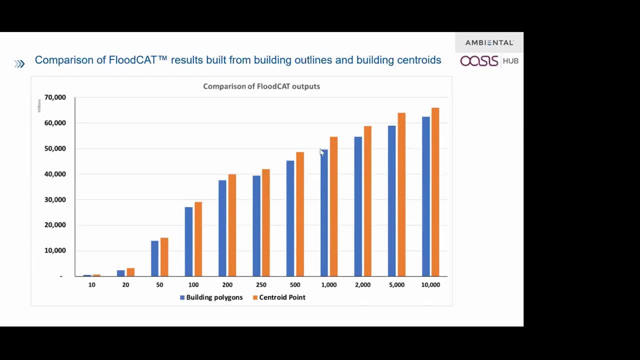 between um flat cat 1, which was produced from building points, and flat cat 2, which was building from building outline. so when we compared these two there was about 10 percentage of risk reduction. this would def well, we are still validating our results, but we can. we can conveniently. 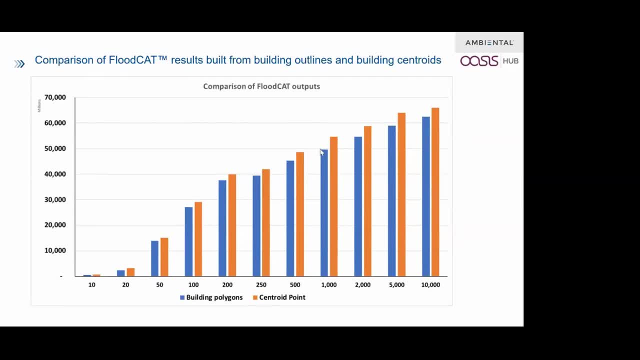 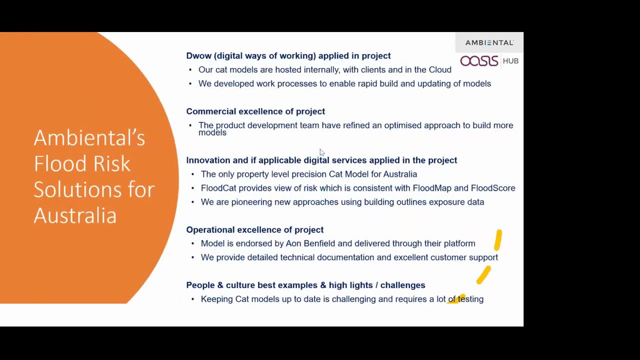 say that using building outlines is having an impact over your overall overall. al's next slide, please. so here's a slide which talks about our salient features, of how we have um, we have implemented our um, our flat cat, and i did mention about producing two different and comparing two. 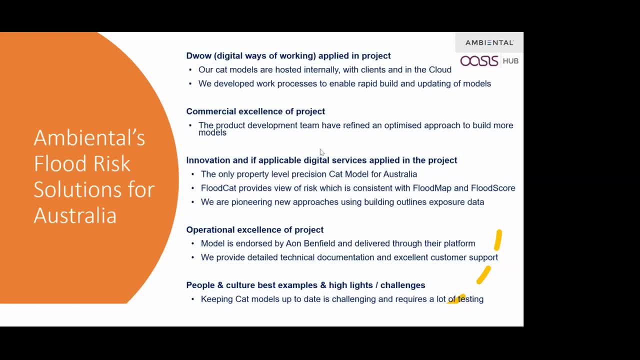 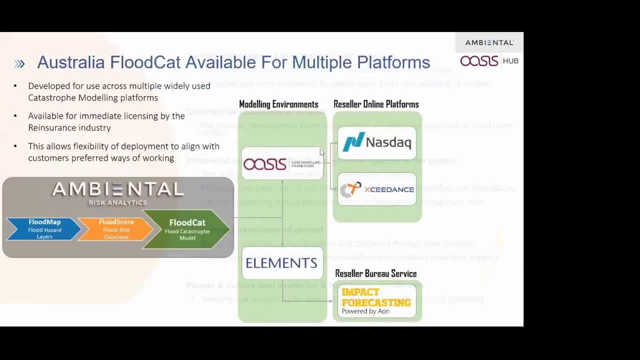 different flat cats. so this means, like we are, we have refined our rapid development and we have automated most of our steps in a flat cat production. next slide, please. so here's the platform where we have deployed our flat cat model. so one is the earth's, which is 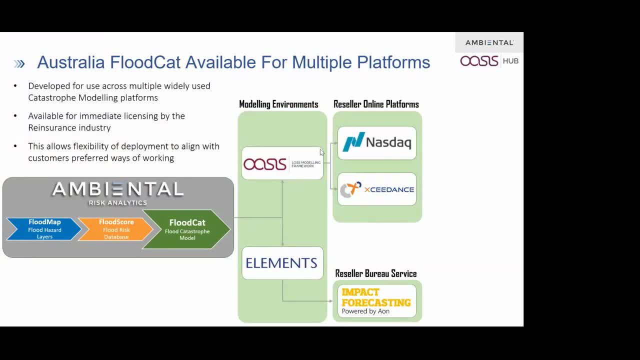 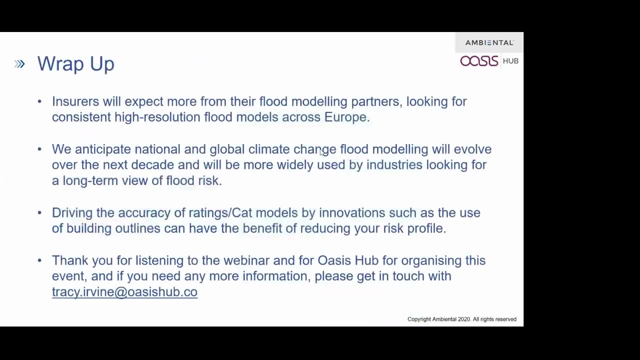 which i'm sure all of you know, uh, and the other one is impact, um, by impact forecasting, which is the elements. thank you very much, excellent. thank you very much, rabini. uh, katie and dave. that's uh three excellent presentations. now just really just to wrap up before we go to questions. um, i think 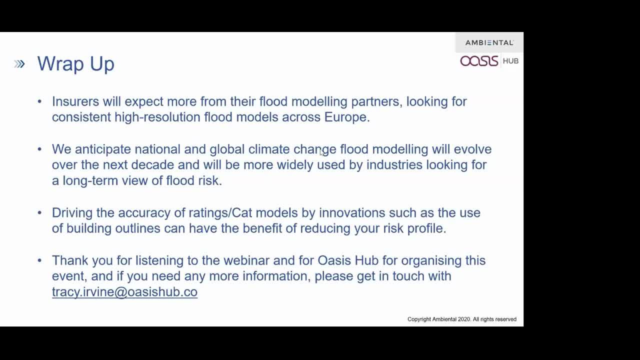 you know, as katie and everybody said, insurers will expect more for their flood models. we're familiar with more and more, i think, with the future of climate change and other sort of improvements in data, insurers and other financial sort of institutions are going to expect more across their flood models. 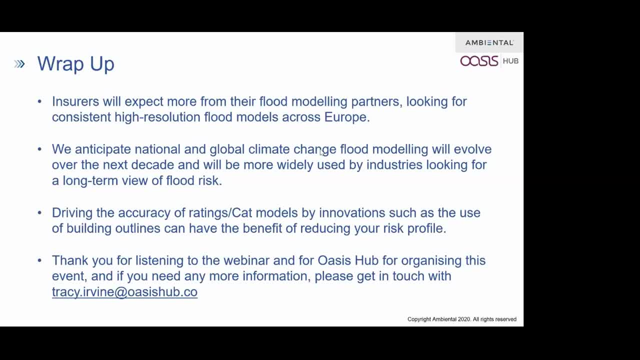 uh high resolution quality of the data across europe and globally. um, we're also experiencing very much on the climate change. um, it's quite early days still, but we're finding that utility companies, local governments, uh insurers and others are all starting to look at climate change, particularly when they have assets which they want to sort of assess in the future. and, as dave, 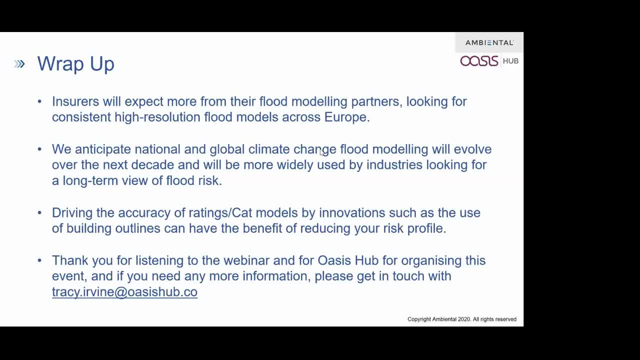 said: um, some of the issues and some of the the models actually strike up a massive increase in, particularly blue, your flooding and others. uh, in the future, um, you know, 30 to 50 years ahead. uh, with the cap models we're really sort of innovating that very much in the market in. 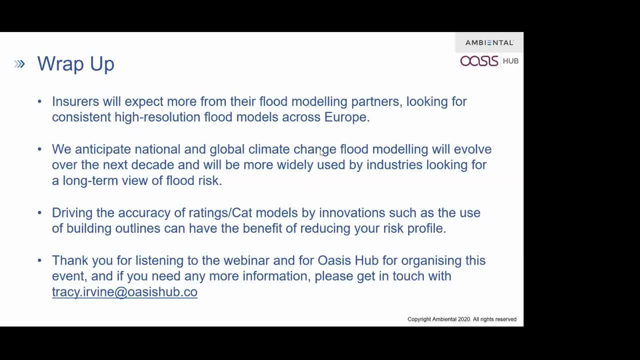 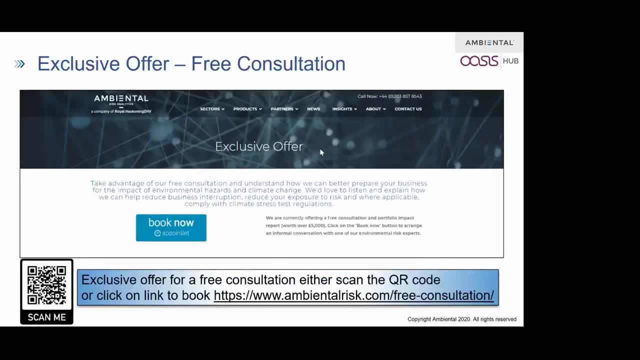 the marketplace with australia and we're looking to develop other models as well. uh, and how we innovate and how we um sort of build those models going forward. um, we had a question- i think it's directed at um david, um or katie, asking how defensible the rainfall discharge for a 10 000 year return period event. 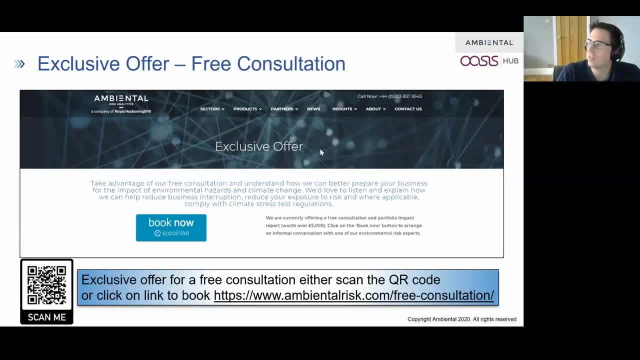 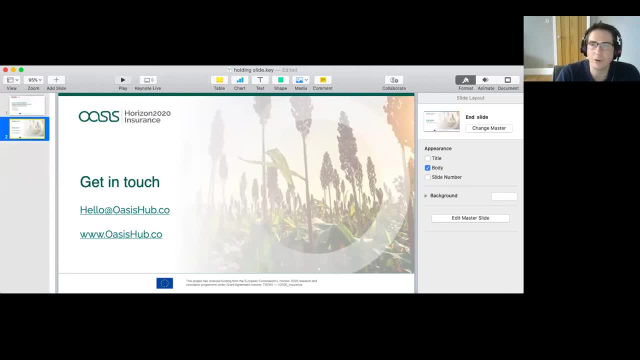 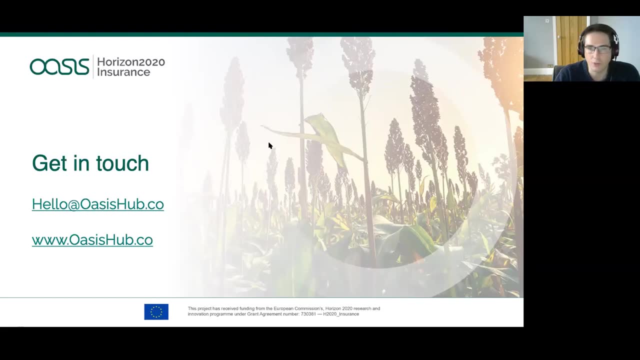 um was. so, yeah, it's a really important question because it it clearly is highly uncertain at that level, um, hydrologically speaking. clearly, you know, we've got nowhere near a 10 000 year uh record to use to predict the the future, um, whether that's climate change or current present day. whatever we do, 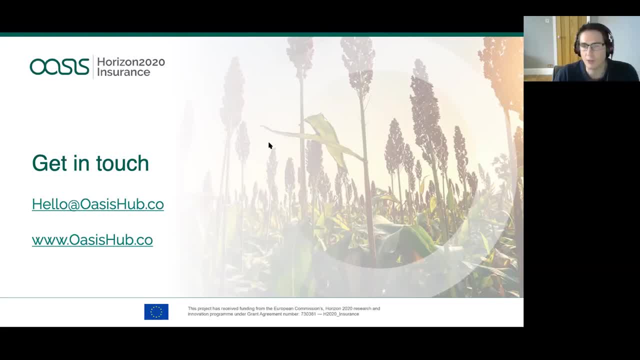 it's very, very uncertain. um, what i would say is defensible is the reason that we do it, um rather than uh. specifically i'll come to that and say: i mean, basically, the reason we need it is for cameras, um, generally, for a full catastrophe model event set. you will. 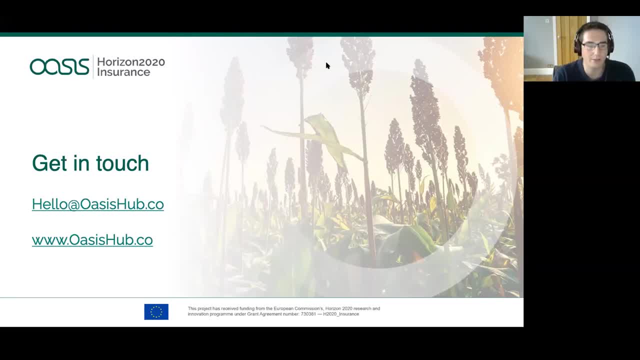 simulate 10 000 years of synthetic weather. that's the kind of industry standard minimum for the number of synthetic years of um, you know, of raid, of events, of um of weather, um. so within that time you would probably expect, uh, 10 or so, or just under events, to exceed that one in a thousand. 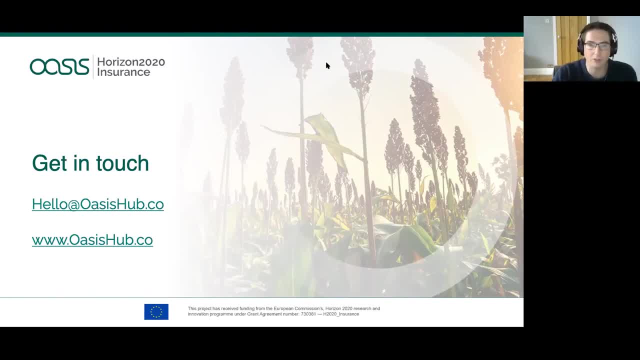 year um return period at certain locations across the country. so, essentially, if you, if you don't have anything beyond the one in a thousand year, which is generally the highest you'll see in, uh, you know, on planning, uh kind of these kind of events, so that's the unexpected. so there's a lot of 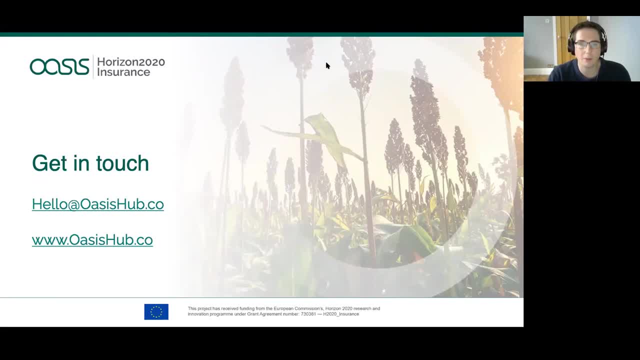 kind of, for example, the Environment Agency planning websites, which in itself is still pretty uncertain, of course, but nothing like 10 times that. If you don't have anything beyond that, then you're essentially guaranteeing that you'll understate those risks. 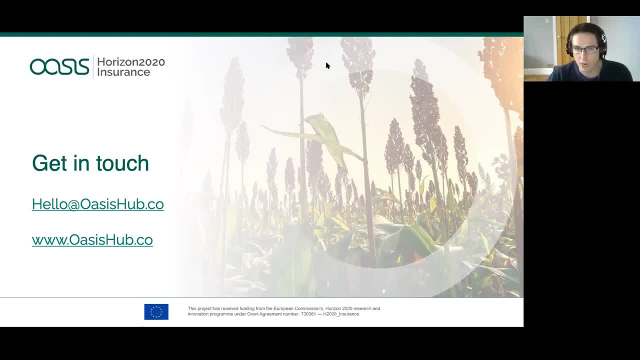 So these ultra-rare events are ultra-rare, but you should, in order to be able to capture the impact that they could theoretically- and we don't obviously experience them very much- occur, we need to have something beyond that level. So that's why we simulate the 10,000-year. It actually barely factors into the insurance risk ratings or the average annual losses because it's too rare. So when you look at the probability side of the equation, it's so low that it can't generate a 1 out of 100 by itself. 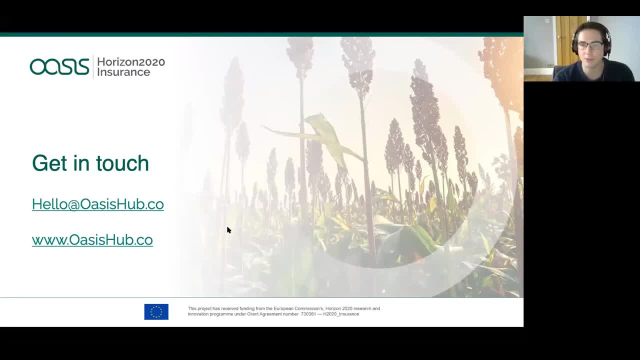 It will flag it as flood-exposed, but it needs to be combined with something that's not a 100.. So we need to have some other logic to actually get onto that scale. David, I think we've got another question for you from Taiwo. 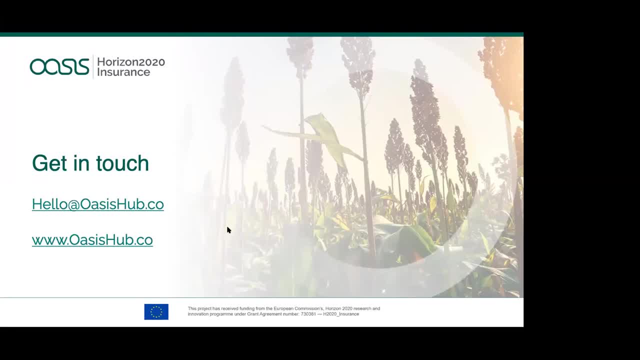 asking what software you use in doing your analysis for the flood mapping. What's the methodology and source of data? So the hydrology is unique to the country. That's one thing we're very keen on. So if we're modelling Spain, we want to use Spanish hydrological methods. 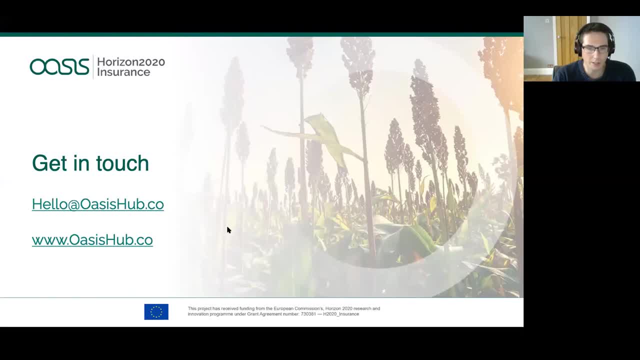 If we're modelling Australia, we use Australian hydrological methods. In the UK- again, UK hydrology- we use Australian hydrological methods or data. Basically, local knowledge tends to be really beneficial when you look at hydrology because if you've been living somewhere, 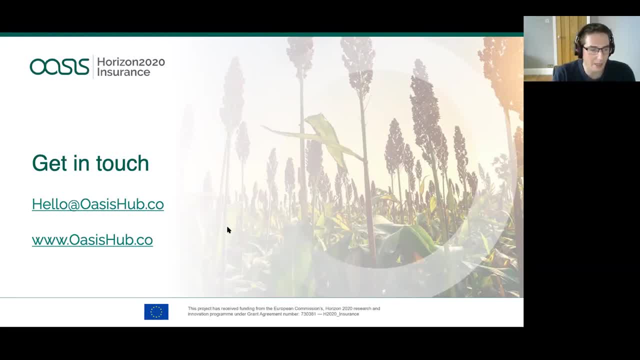 and experiencing these things for a long time, then clearly the engineering manuals are likely to capture that. So that's on the hydrology side. So that varies and that could be from Excel models to more sophisticated hydrological packages. But on the hydraulic modelling, 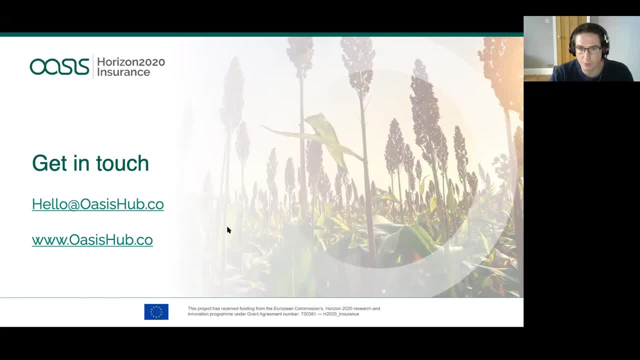 we use our own proprietary system called FLOWROOT, which is a two-dimensional flood model but similar to something like ListBlood or 2FLOW. Basically, it moves water along the UK. In Europe, all of our models are five-metre hydraulic models. 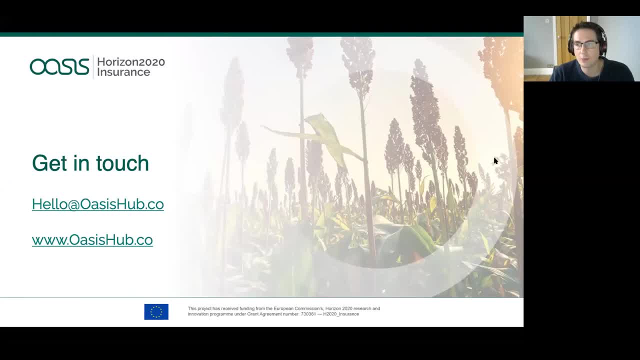 so it has to run very quickly And we're spinning up. you know. put it into context: The UK has more than a million hydraulic flood models simulated, So it's something We have to use our own tools because we need to script them.